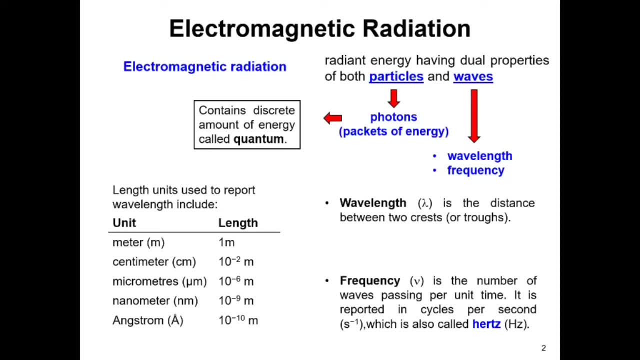 act as a wave because it has wave-like characteristics. It has wavelength and frequency. Wavelength, which has the symbol lambda, is the distance between two crests or two troughs. Frequency, on the other hand, has the Greek letter, symbol nu, which is defined as the number of waves. 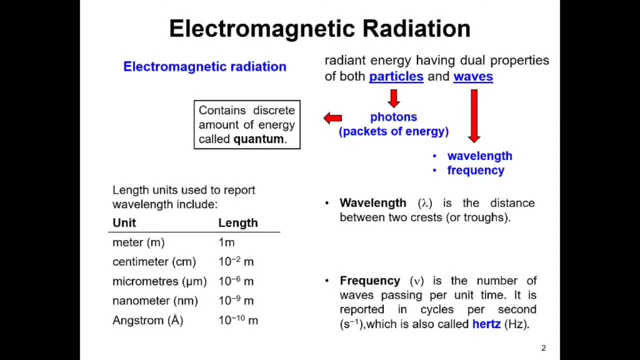 per unit of time. It is reported in cycles per second or inverse second, which is also known as the hertz, And shown here on the left are the different units used to report wavelength, So you can have meter, centimeter, micrometers, nanometer or angstrom. So there's a lot of different types. 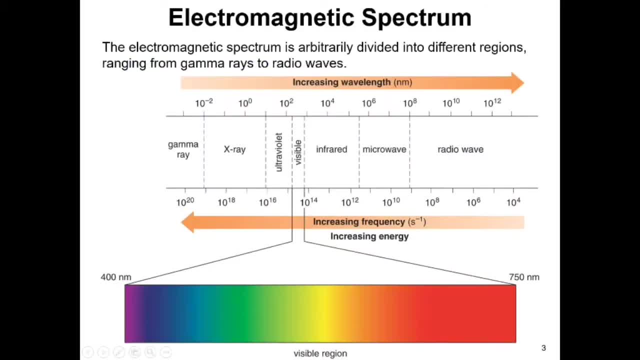 of light because, again, light, by definition, is an electromagnetic radiation, And so radio wave is an example of light because it is an electromagnetic radiation, And so radio wave, microwave, infrared, visible all the way to gamma ray, are all examples of light And they make up the 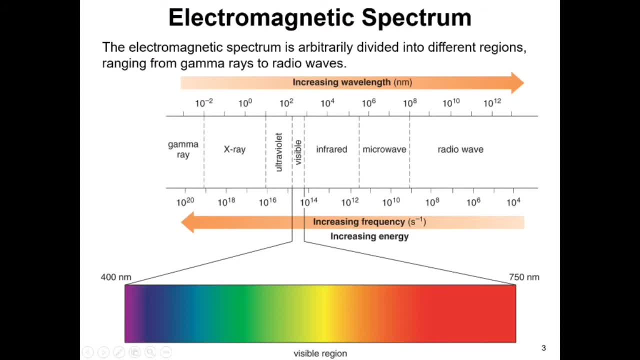 electromagnetic radiation spectrum. So when you look at the visible light, it's actually just a small portion of the electromagnetic spectrum And it ranges from 400 nanometers to 750 nanometers. So they call this the visible region of the spectrum, because the cones in our eyes can only 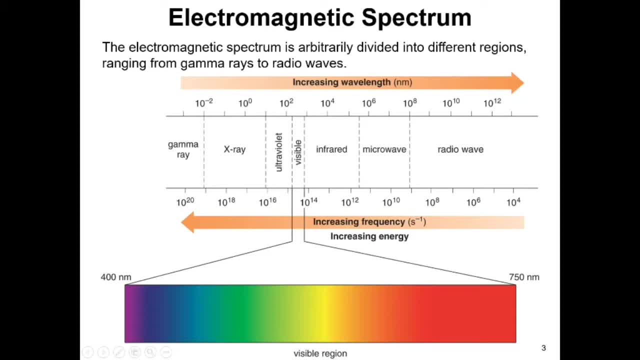 absorb this specific light. So the visible light is a specific region of the electromagnetic spectrum. A lot of proteins can absorb energies in the UV visible region. Other molecules can also absorb in the near infrared region. That's why IR spectroscopy uses infrared light to distinguish the different bonds present in the 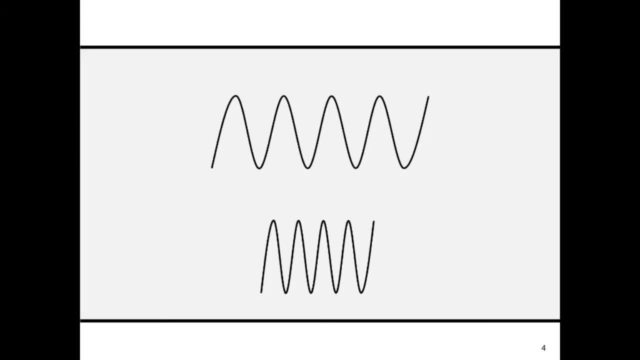 chemical structure. So we know that light is a wave And its energy can be described by a mathematical wave function, as shown here. A wave has three different characteristics: A wavelength, frequency and amplitude. Here we have two different waves with two different wavelengths. 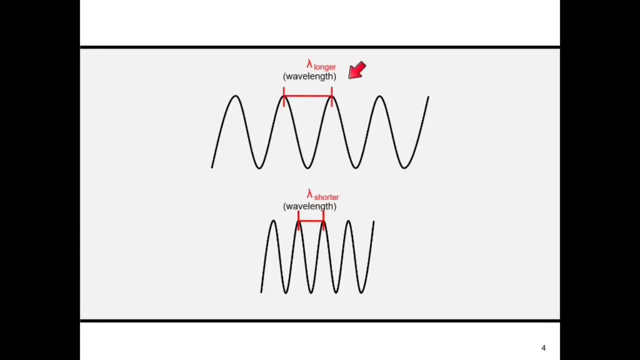 and frequencies. The wavelength is measured as a distance between two peaks, as shown here. So here we have the longer wavelength and at the bottom we have the shorter wavelength. On the other hand, frequency is defined as a number of cycles per second. So here you can see that the wave up top. 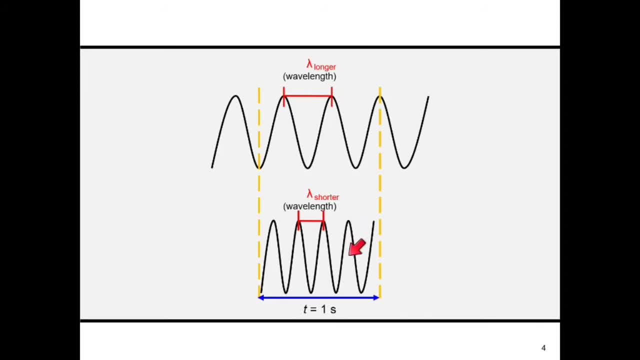 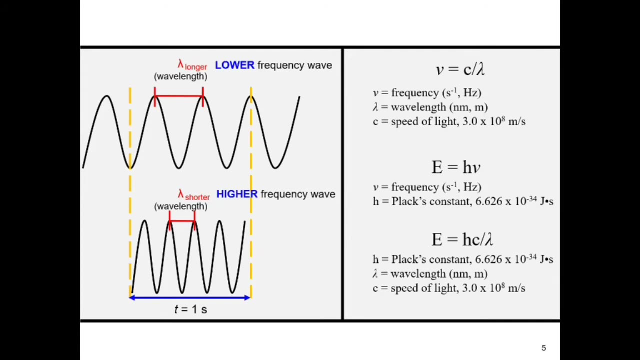 has a lower frequency compared to the wave at the bottom. So we have lower frequency wave here and a higher frequency wave. So here you can see that wavelength, frequency and energy are all related mathematically. The first equation here relates frequency and wavelength. So frequency is equivalent to the speed of light. 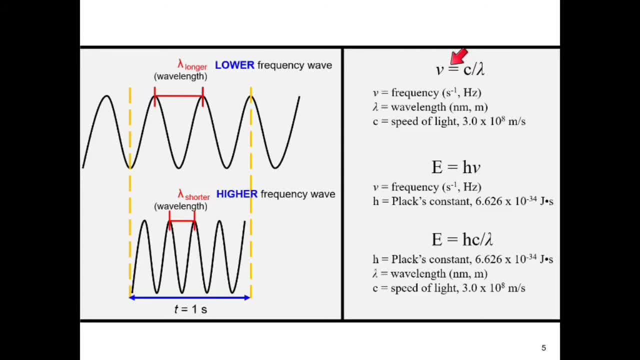 divided by the wavelength And frequency is measured in inverse second or hertz. Speed of light is measured in meters per second, and this is a constant. So three times ten to the eighth. power And wavelength is measured in either nanometers or meters. So here you can see that wavelength, 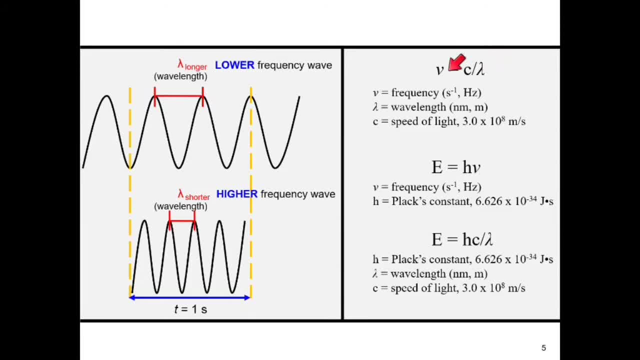 is inversely related to the frequency, And so as the wavelength increases, the frequency decreases and vice versa. And the second equation here relates energy and frequency, And so energy is equivalent to Planck's constant times frequency. Again, frequency is measured in hertz, or inverse. second, And Planck's constant 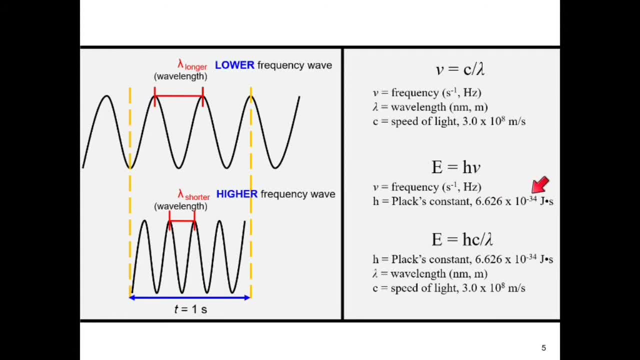 is equivalent to six point six, two, six times ten to the negative thirty-fourth power joules seconds. So in this equation you can see that energy is directly proportional or directly related to the frequency of the wave, And so as the frequency increases, so does energy. So here you can see that equation number one can be substituted. 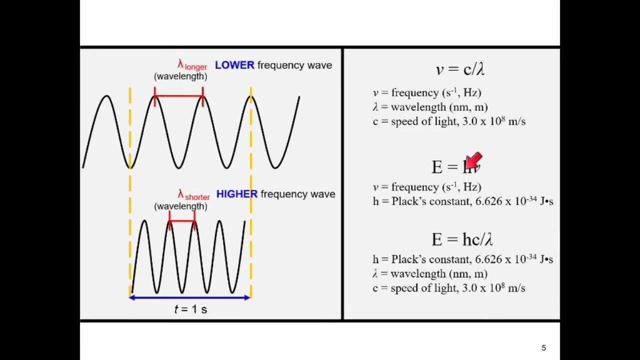 into equation number two, And what we get is the second equation for energy, And this relates the wavelength and the energy of the wave. So E is equivalent to Planck's constant times, the speed of light divided by wavelength. And so in this equation you 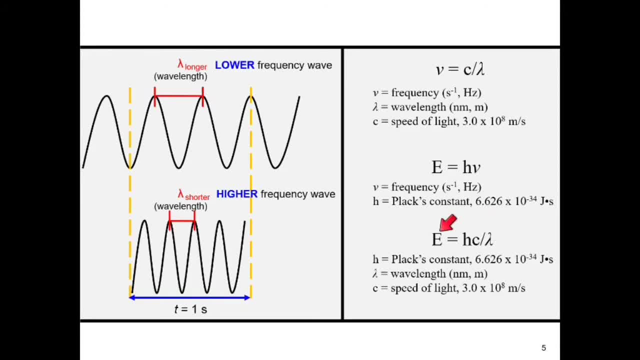 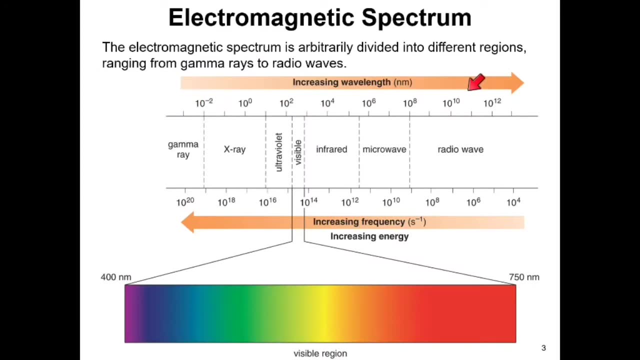 can see that wavelength is inversely proportional to the energy, And so the longer the wavelength, the lower the energy, And the shorter the wavelength, the higher the energy. So here's the electromagnetic spectrum again. You can see that wavelength is up top and frequency is at the bottom, And so you can see that. 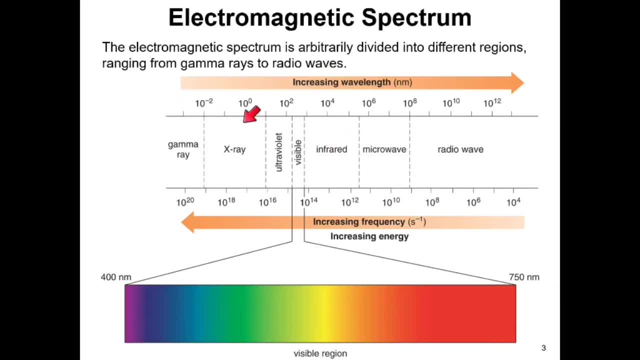 wavelength increases from left to right, So from gamma ray all the way to radio wave, And then frequency is inversely related to the wavelength, And so frequency increases in the opposite direction, from right to left In terms of energy. energy increases with frequency. 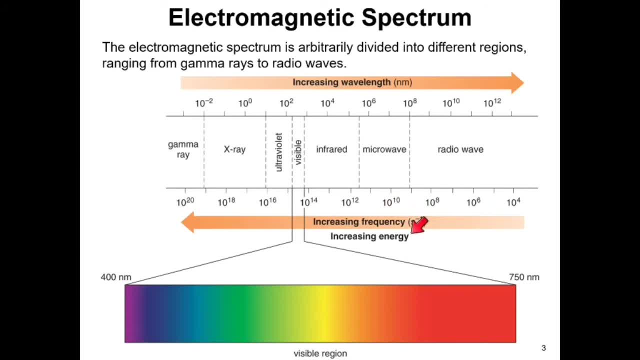 And so that means that energy will also increase from right to left. And so in that case, when you look at the different regions of the spectrum, the gamma ray here has the highest energy and frequency, But it has the shortest wavelength. On the other hand, radio wave 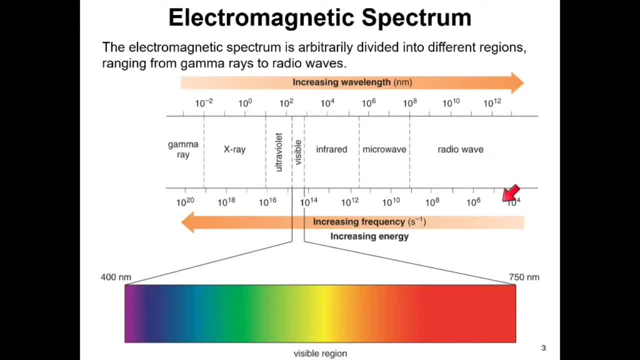 has the longest wavelength but shorter frequency or lower frequency and energy. And so, looking at the visible region of the spectrum, you can see that purple or blue light here has the shortest wavelength, whereas red light has the longest wavelength And so red has a lower energy and frequency compared to the purple light. 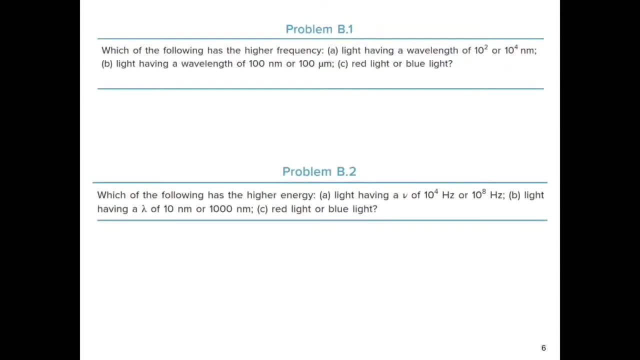 So here's practice problem number one: Which of the following has the higher frequency: Light having a wavelength of 100 nanometers or 10,000 nanometers? So, in terms of frequency, wavelength is inversely related to frequency, And so the higher the frequency, the lower or the 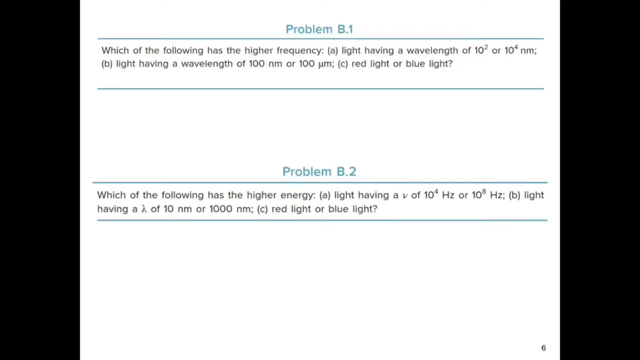 shorter the wavelength, And the longer the wavelength, the lower the frequency, And so in that case the shorter wavelength would have a higher frequency. What about part B? here It says light having a wavelength of 100 nanometers or 100 micrometers. So again, the higher the frequency. 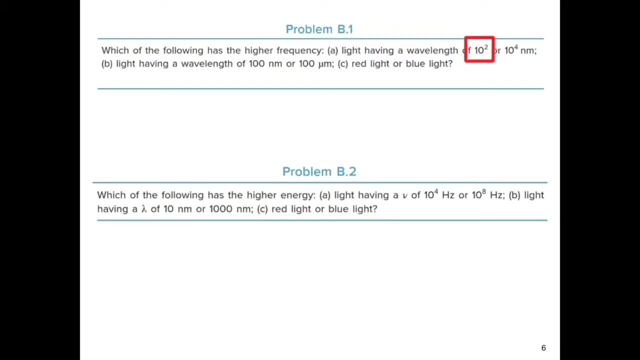 the shorter the wavelength, And so, in this case, 100 nanometers would have a higher frequency. And finally, red light versus blue light In terms of frequency: the shorter the wavelength, the higher the frequency, And so blue light has a shorter wavelength, around 400 nanometers. 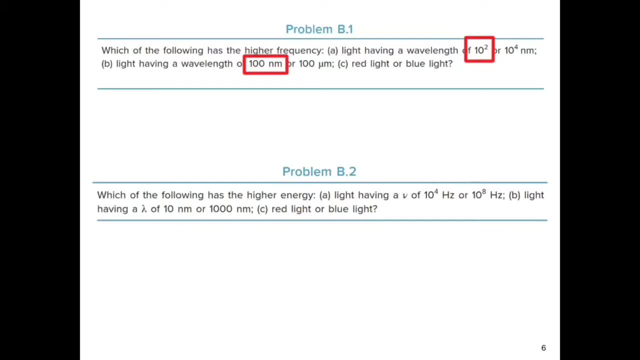 whereas red light has a higher and longer wavelength in around 750 nanometers. And for the second problem here, which of the following has the higher energy: Light having a frequency of 10 to the 4th hertz or 10 to the 8 hertz. So, in terms of energy and 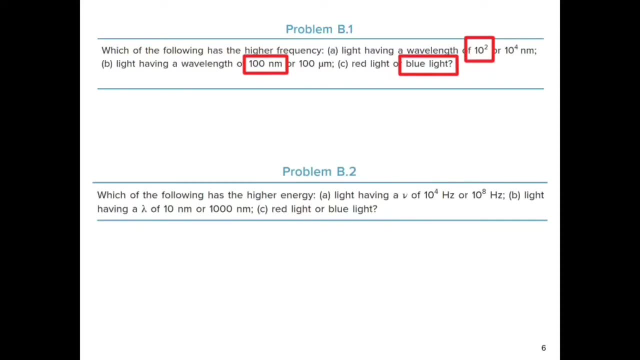 frequency. they are directly related And so the higher the energy, the higher the frequency. So in this case, 10 to the 8th hertz would have a higher energy. What about light having a wavelength of 10 nanometers or 1,000?? 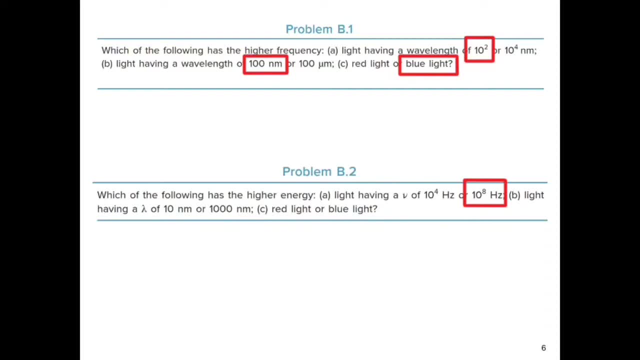 Of course, that's another answer, And it is important to note that the match don't have an energy balance with the드� dú above the wave length, And so that could be aốc potencialitte feed fio ng hybrid range. 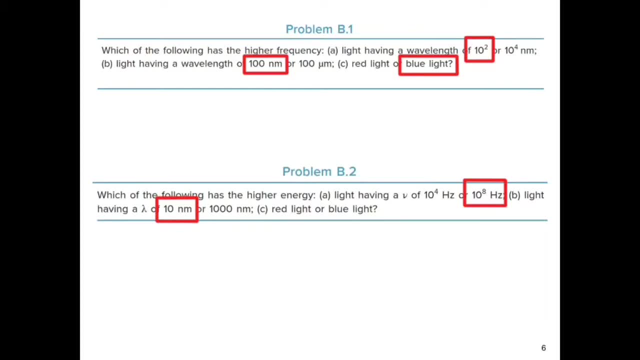 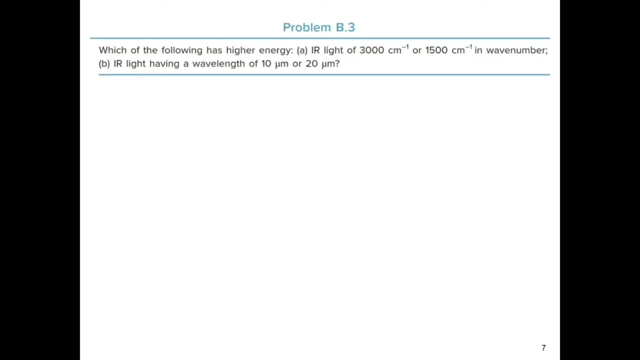 g, fio, ng hybrid group universities. higher energy than the red light. And here's practice problem number three: Which of the following has a higher energy? IR light with 3000 inverse centimeter or 1500 inverse centimeter? And so, before we can answer this question, 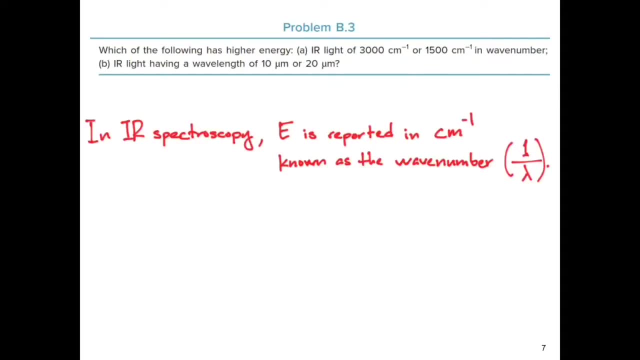 one thing that you need to know is that in spectroscopy, in IR spectroscopy, energy is reported in inverse centimeter, And this is also known as the wave number, And this is essentially the inverse of a wavelength, one over the wavelength. 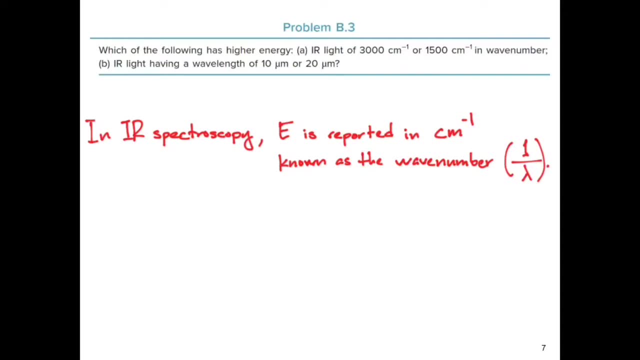 And so because of that, the higher the wave number, the higher the energy, And the smaller the wave number, the lower the energy. So now for part A. here it says: IR light of 3000 wave number or 1500 wave number. 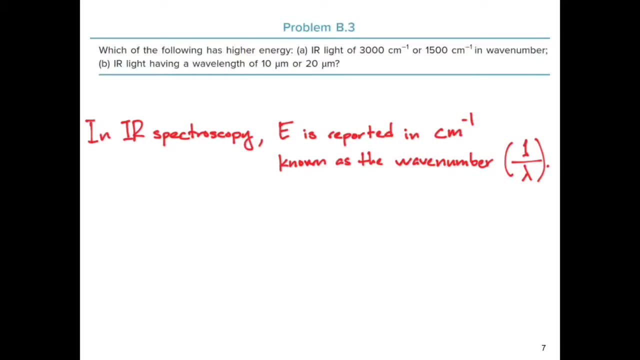 Which one has the higher energy. Well, wave number is directly related to energy, And so 3000 inverse centimeter would have the higher energy. And for the second part here, IR light having a wavelength of 10 micrometers or 20 micrometers. 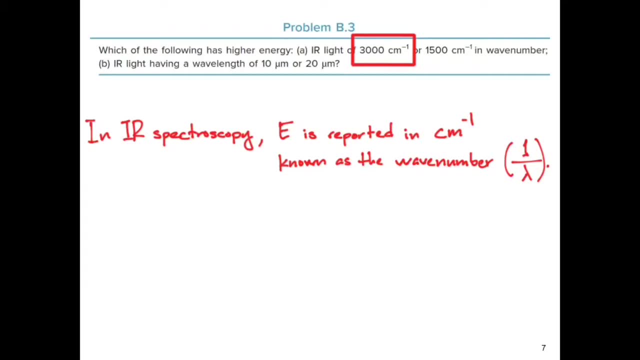 So this is again wavelength And so that don't get wavelength confused with wave number. So in terms of wavelength and energy, wavelength is inversely proportional to energy, And so the longer the wavelength, the lower the energy. The shorter the wavelength, the higher the energy. 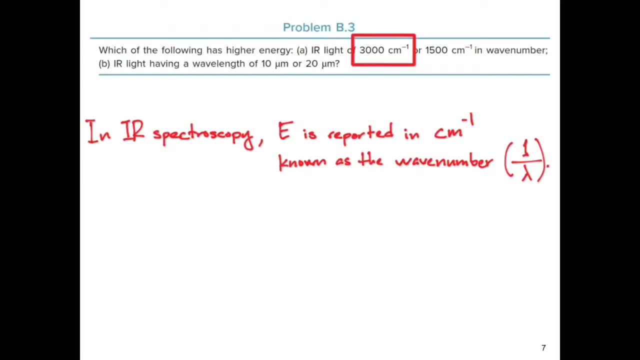 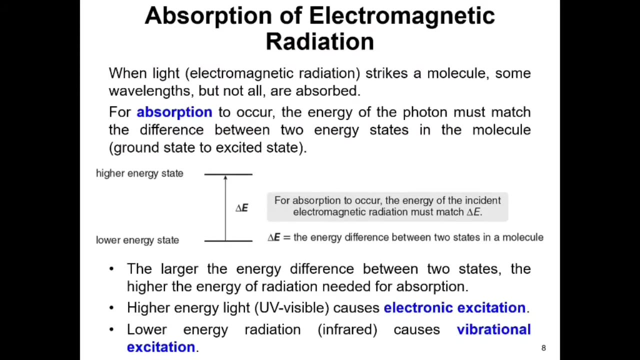 So 10 micrometers is shorter than 20 micrometers, And so you would have a higher energy. So at the beginning of this video I mentioned that molecules interact with light. They can either absorb light or transmit light When light, which is electromagnetic radiation. 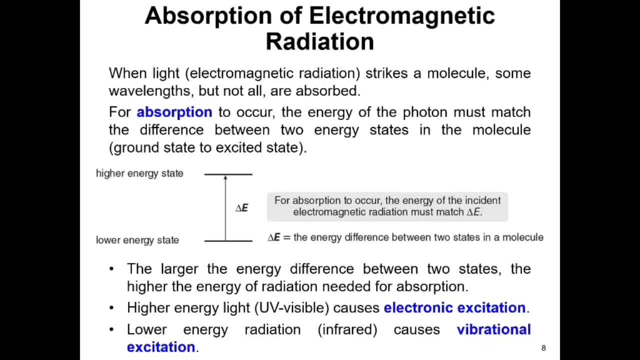 strikes a molecule, some of the wavelengths or energies are absorbed, And so the energy is absorbed, And in order for this absorption to happen, the energy of the photon has to match the energy of the bonds within the given molecule, And this is the difference between two energy states. 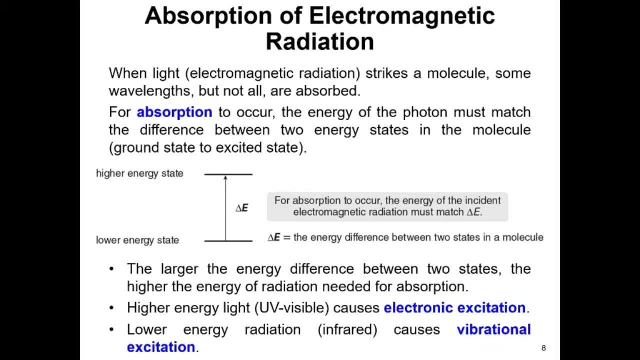 in the molecule ground state to excited state. Ground state is the lower energy level And the excited state is the higher energy level And the difference between them in terms of energy is delta E, And the larger this delta E is, the higher the energy of radiation needed for absorption. 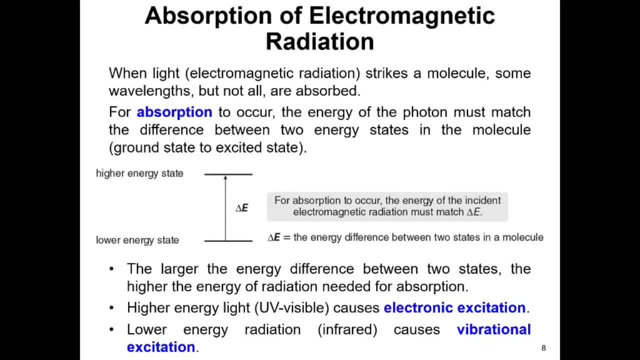 And so in infrared spectroscopy a larger delta E means larger wave number. Higher-energy light, such as the UV visible region, causes electronic excitation, whereas lower energy radiation, such as infrared or near-infrared, causes vibrational excitation. 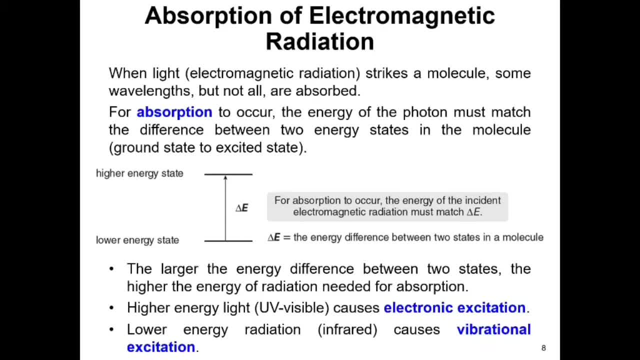 In infrared spectroscopy we only care about vibrational excitation. So in general chemistry you learned a little bit about quantum mechanics. You learned about the principal energy levels and these principal energy levels- levels- are essentially the vibrational energy levels. 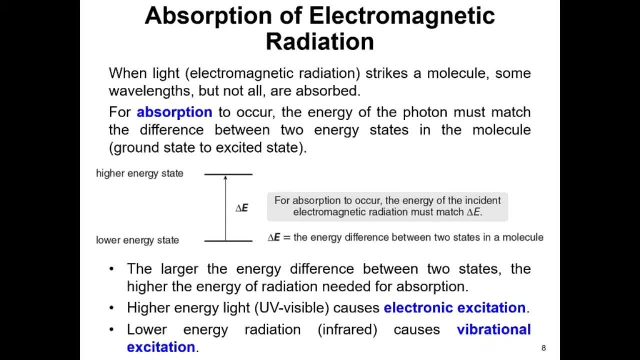 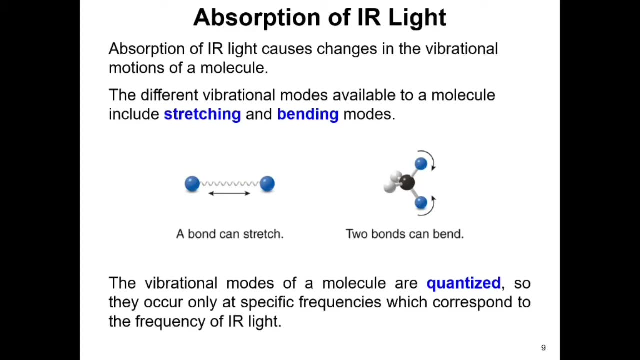 And so when an electron jumps from the ground state to a higher energy level, we call that an excitation, And if it involves vibrational energy levels, then we call that vibrational excitation. So when a molecule absorbs infrared light, it causes changes in the vibrational motions. 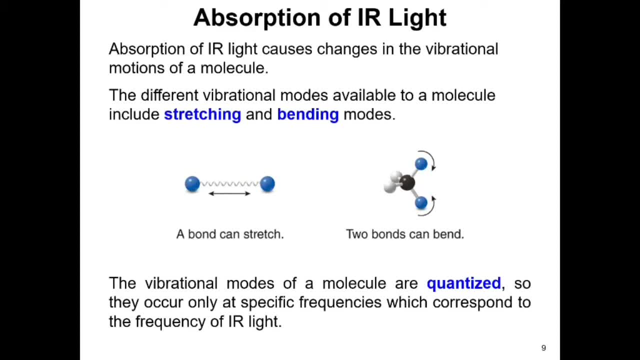 And these vibrational motions are stretching and bending. So a bond can stretch and bend. So the energies of the vibrational modes of a molecule are quantized. So that means that they occur only at specific frequencies which correspond to the frequency of infrared light. 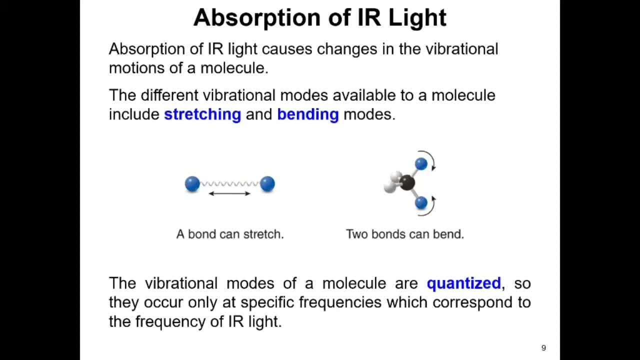 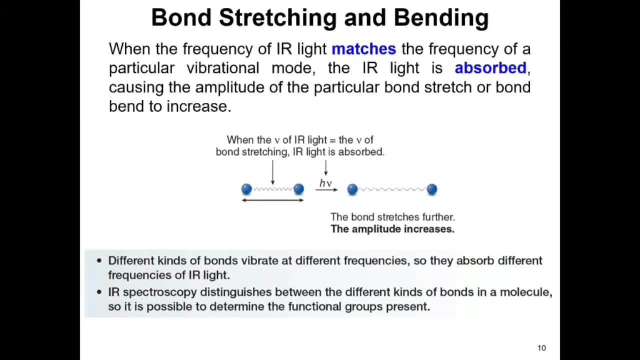 So the change in energy associated with these vibrational motions within a molecule has to match the frequency or the energy of the infrared light. So when the frequency of infrared light matches the frequency of a specific vibrational mode, the infrared light is absorbed And this causes the amplitude. 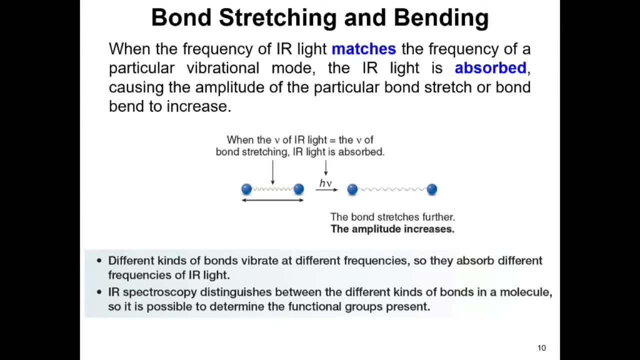 of the particular bond stretch or bond bend to increase. So here you can see that we have two atoms that are connected via a chemical bond, And so when this bond stretches, it corresponds to a specific energy, And so when this energy matches the energy, 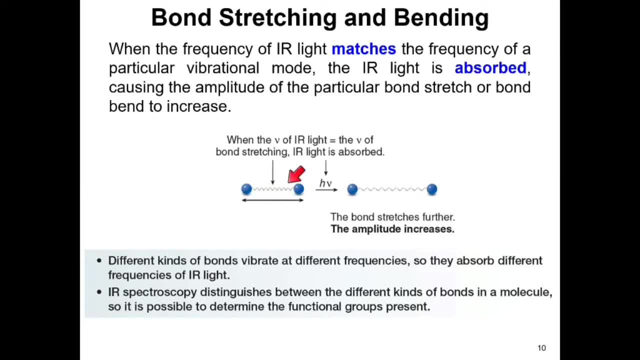 of the infrared light, then that infrared light is absorbed And that absorption causes the amplitude to increase, And again, in infrared spectroscopy this is detected, And so different kinds of bonds vibrate at different frequencies, And so that means that they absorb at different frequencies. 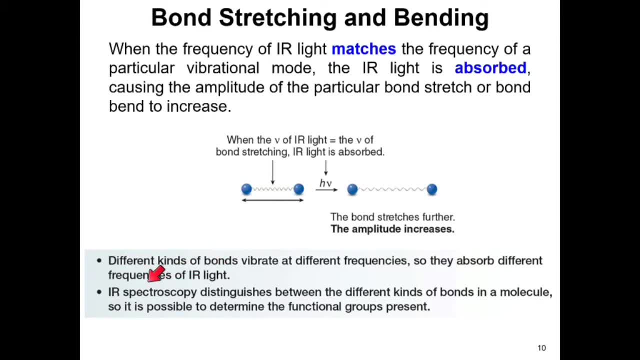 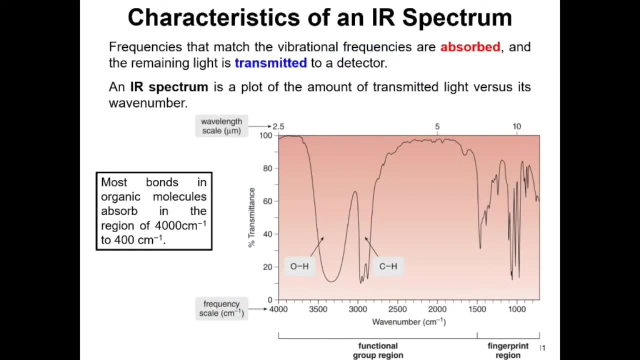 or energies of infrared light, And so we can use IR spectroscopy to differentiate between the different kinds of bonds within a given molecule, And this allows us to basically determine the different functional groups that are present in a given capital structure. So this is what an IR spectrum looks like. 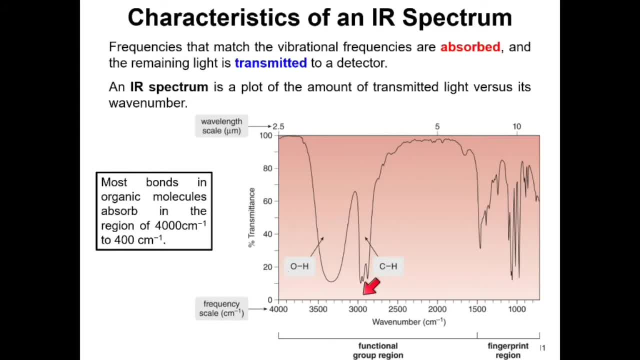 We have the percent transmittance on the y-axis and the wave number in the x-axis. Percent transmittance go from 100% all the way down to 0% And this tells us how much of the infrared light was absorbed or transmitted at a specific wave number. 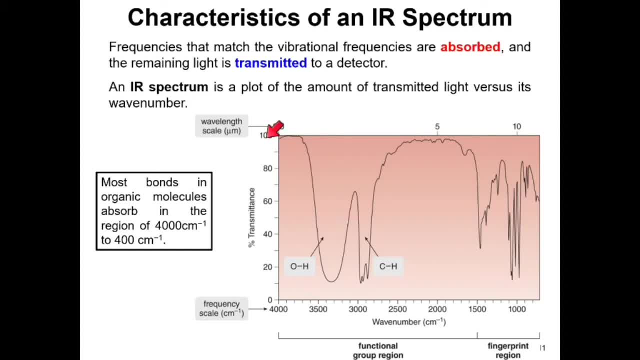 So 100% transmittance tells us that none of the infrared light was absorbed at that specific wave number, And 0% transmittance tells us that 100% of the light was absorbed at that specific wave number. And on the x-axis we have the wave number. 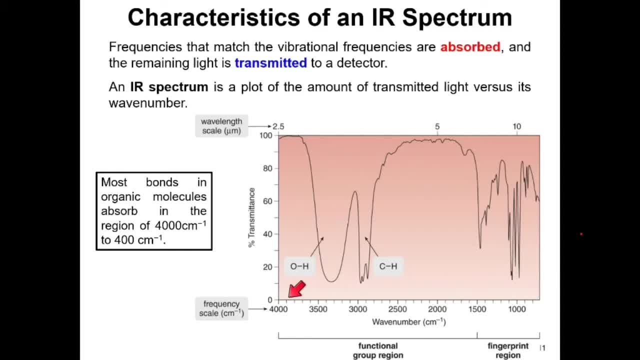 And it ranges between 400 wave number all the way to 4,000 wave number. And remember that the higher the wave number, the larger the frequency and the energy. So all of these sharp lines here, including this broad curve, here, these are known as peaks. 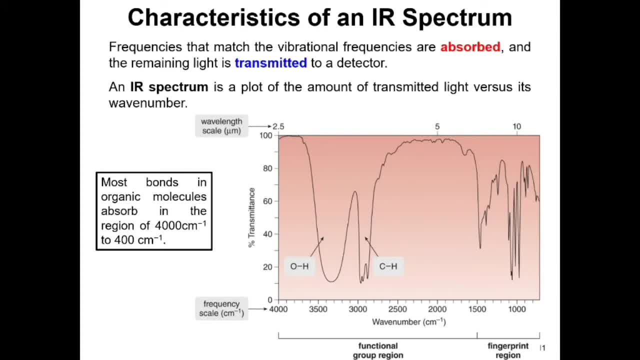 They're known as characteristic peaks, And these peaks correspond to a specific energy of the infrared light that was absorbed by that specific bond within that given molecule. And so, for example, here we have a characteristic peak coming from an oxygen molecule. And so, for example, here we have a characteristic peak coming from an oxygen molecule. 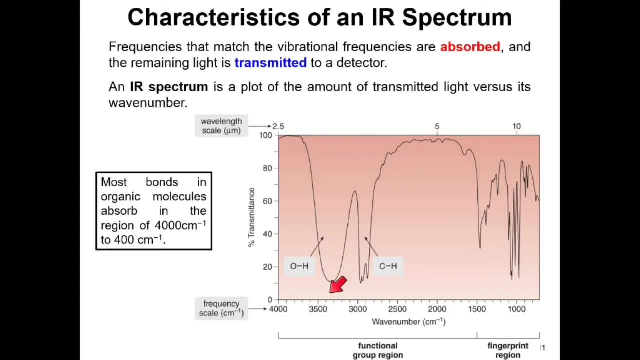 here we have the carbon-to-hydrogen bond, which occurs at about 3,300 wave number, which occurs at about 3,300 wave number, And here we have the carbon-to-hydrogen bond that occurs below or between 2,800 and 3,000 wave number. 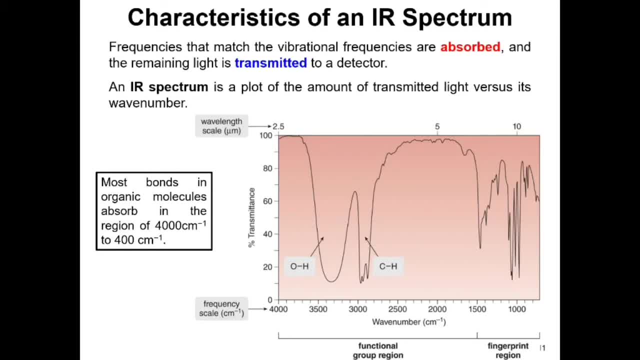 And so these are characteristic peaks which correspond to a specific bond within a given molecule. So every IR spectrum contains two main regions: the fingerprint region and the functional group region. In this video we're only going to focus on the latter, which is the functional group region. 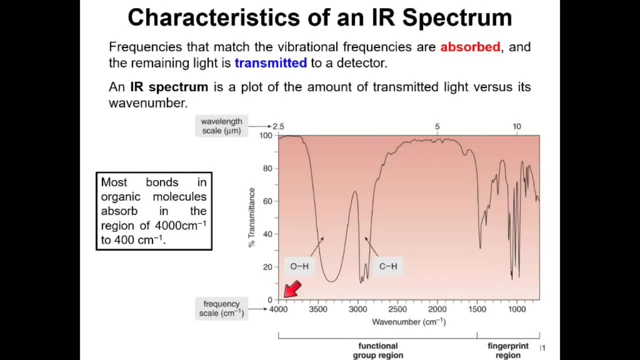 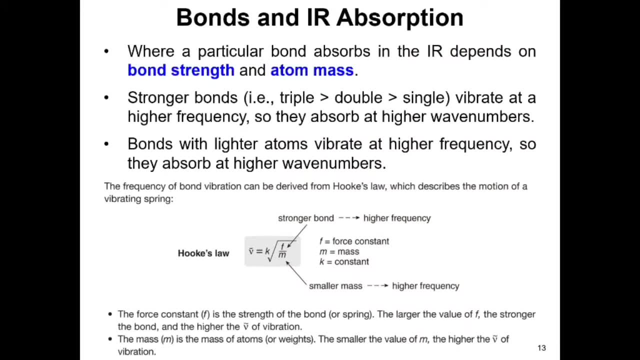 which occurs between 1500 wavenumber and 4000 wavenumber. So the amount of energy that the bond absorbs will depend on two things: the strength of the bond and the mass of the atoms involved in that bond. Stronger bonds will vibrate at a higher frequency and so they will absorb at higher wavenumbers. 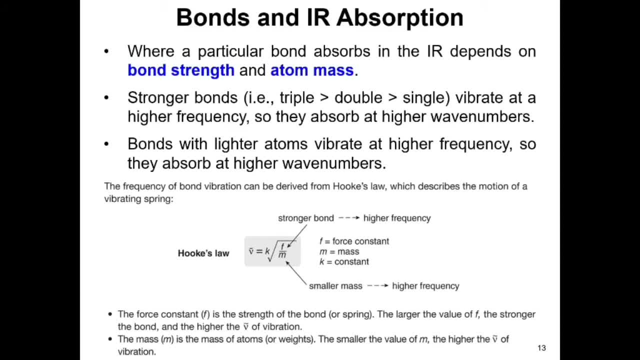 So you would expect a carbon-carbon triple bond to absorb at a higher wavenumber compared to a carbon-carbon double bond or a carbon-carbon single bond. Bonds with lighter atoms will vibrate at a higher frequency as well, and so they will absorb at higher wavenumbers. 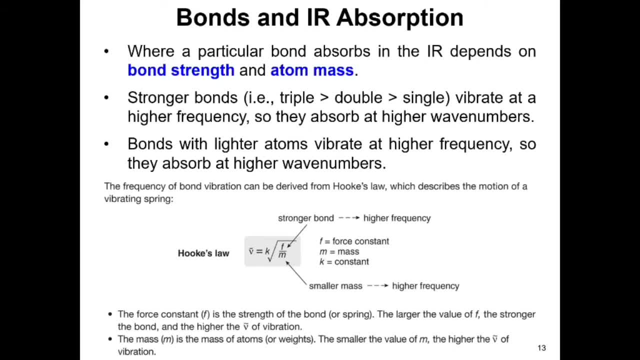 The greater the difference is in the atomic masses, results in the vibration at a higher frequency and the absorption at higher wavenumbers. So the frequency of bond vibration can all be derived from Hooke's law, which describes the motion of a vibrating spring. 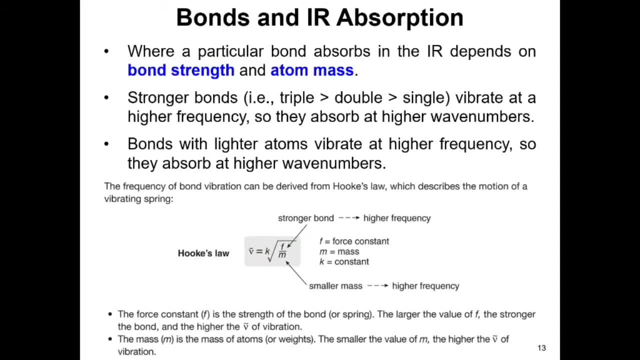 And it's all summarized in this equation, as shown here. So in this equation you can see that the frequency is directly proportional to the strength of the bond, but inversely proportional to the mass, And so the stronger the bond, the higher the frequency. 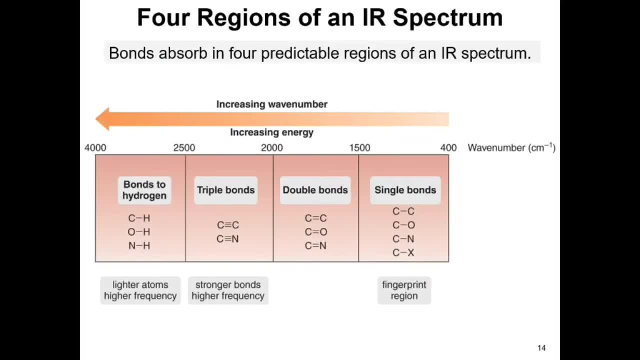 The smaller the mass, the higher the frequency. An IR spectrum has four predictable regions. We have the single bonds, double bonds, triple bonds and bonds to hydrogen. In an IR spectrum, wavenumber increases from right to left, from 400,. 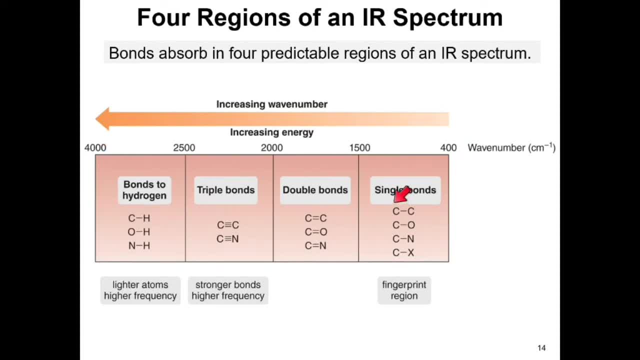 to 4,000, wavenumber. Single bonds occur between 400 and 1500 wavenumber and they call this the fingerprint region. The functional group region ranges between 1500 to 4,000 wavenumber and this can be subdivided into three groups. 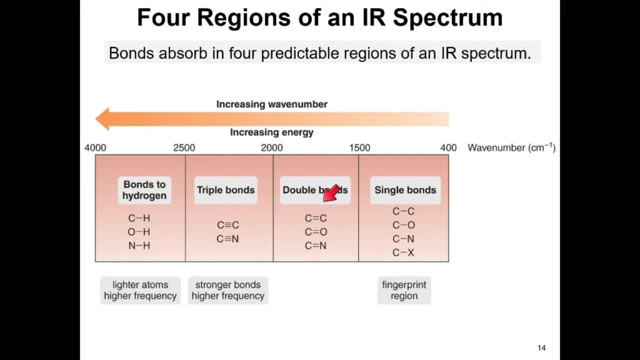 Again the double bonds, triple bonds and bonds to hydrogen. Double bonds occur between 1500 to 2000 wavenumber, triple bonds occurred between 2,000 and 2,500 wavenumber And bonds to hydrogen occur between 2500 to 4000 wavenumber. 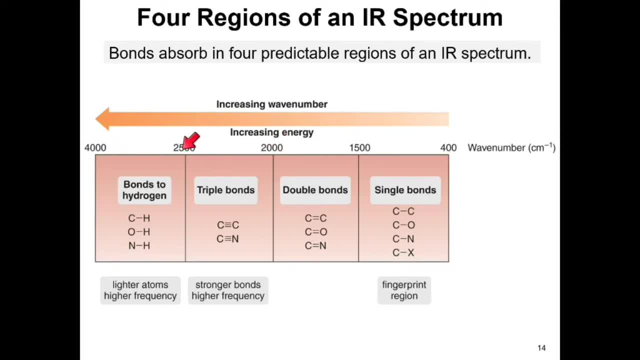 So here you can see that triple bonds occur between 2000 and 2500, and these triple bonds are the stronger bonds which occur at higher frequency. Lighter atoms also occur at higher frequency, such as the carbon to hydrogen bond, oxygen to hydrogen bond and nitrogen to hydrogen bond. 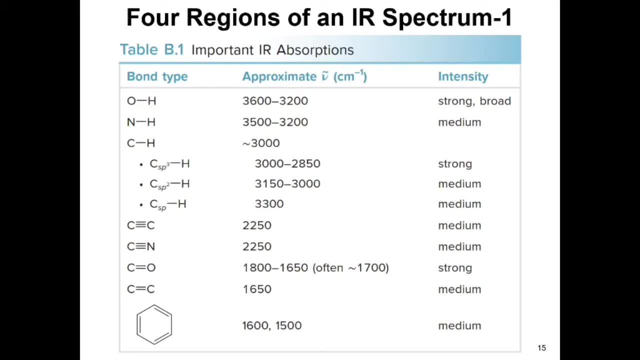 So here's the table that basically summarizes some of the most important IR absorptions. So here at the top we have single bonds involving hydrogen atoms. So we have oxygen to hydrogen bond, nitrogen to hydrogen bond and different types of carbon to hydrogen bonds. 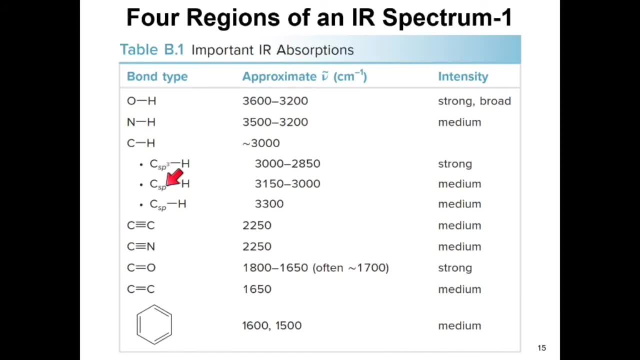 We have sp-hybridized carbon to hydrogen bond, sp2-hybridized carbon to hydrogen bond and sp3-hybridized carbon to hydrogen bond. So you can see that all of these single bonds involving hydrogens occur between 2850 and. 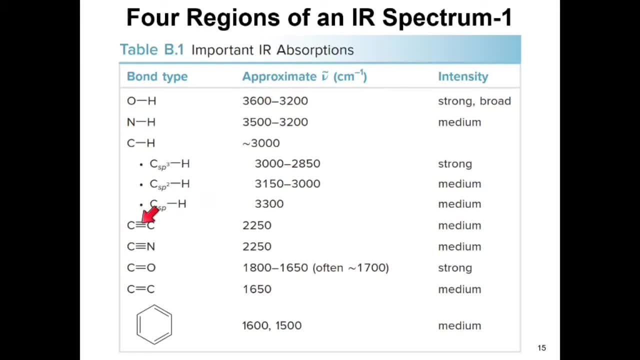 3600.. And here you can see that carbon to carbon triple bond, as well as carbon to nitrogen triple bond, Carbon to oxygen triple bond, occur around 2250 wavenumber. Carbon to oxygen double bond, which is a carbonyl group, occurs around or between 1650 to 1800. 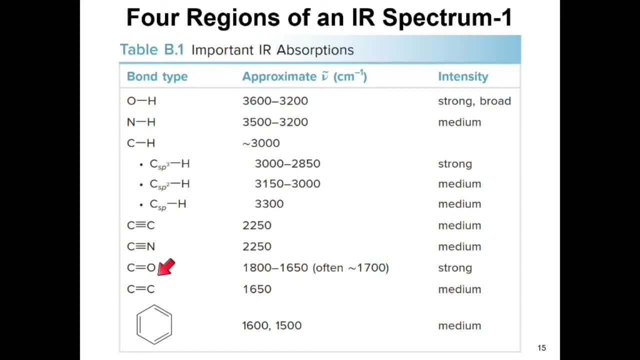 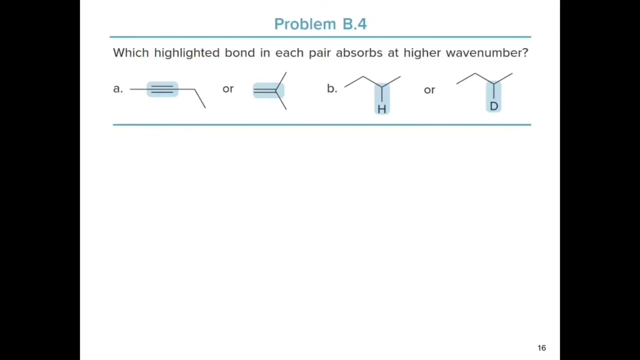 On average it's about 1700.. A carbon-carbon double bond occurs around 1650 wavenumber. A benzene ring occurs between 1600, or you'll see two peaks at 1600 and 1500.. So here's practice. problem number four: 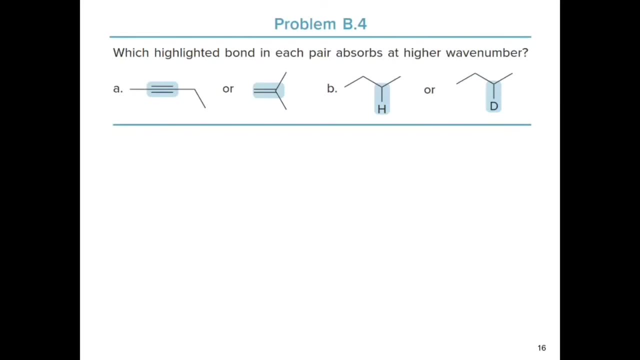 Which highlighted bond in each pair absorbs at a higher wavenumber. So for the first one here you can see that we have a triple bond versus a double bond, And so, because a triple bond is a stronger bond, it will absorb at a higher wavenumber. 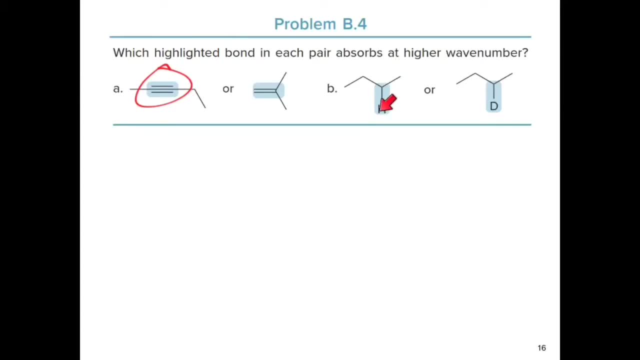 And for part b. here we have a carbon to hydrogen bond versus a carbon to deuterium bond. Since carbon to hydrogen, Since hydrogen is a lighter atom compared to deuterium, You would expect carbon to hydrogen bond to absorb at a higher wavenumber. 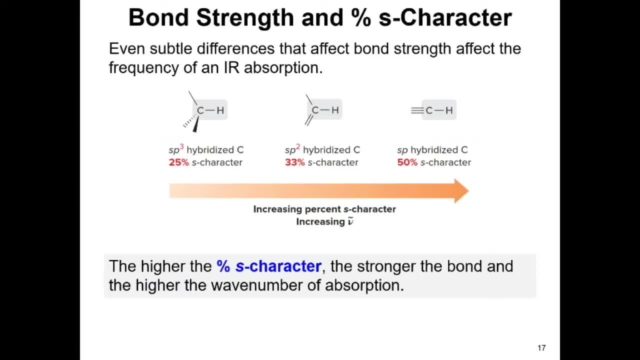 The hybridization of a bond can affect the strength of a bond and therefore can also affect the frequency of an IR absorption. So in one of the earlier chapters you learned that the bond with a higher percent S character is the stronger bond, And so an sp-hybridized carbon to hydrogen bond is stronger compared to an sp2 hybridized. 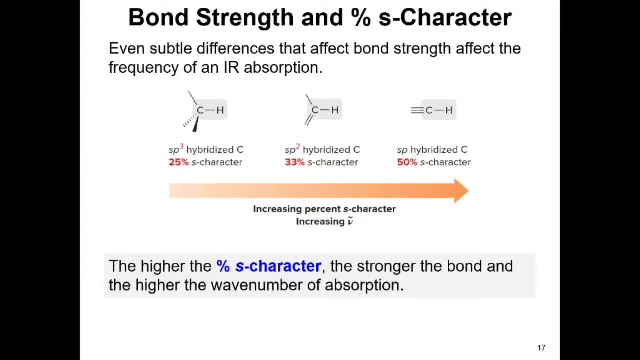 or an sp3 hybridized, And so you would expect an sp-hybridized carbon to hydrogen bond to absorb at a much greater wavenumber. And so here, the higher the percent S character, the stronger the bond and the higher the 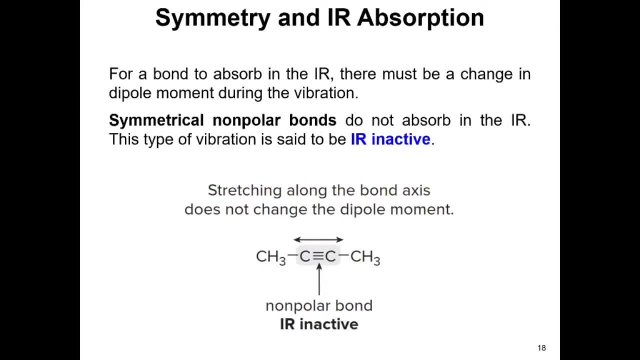 wavenumber of absorption. One important thing that you should also remember is that symmetrical nonpolar bonds do not absorb in the infrared, And this type of vibration is known as IR inactive Or infrared inactive, And so when you look at this molecule here with a triple bond, you can see that this 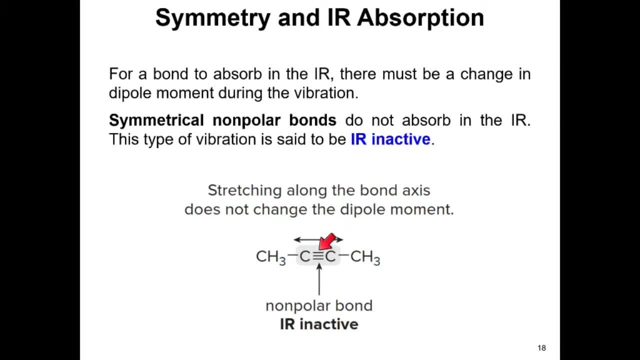 triple bond is a nonpolar bond And therefore this is going to be an IR inactive. You won't see a carbon-carbon triple bond in the 3000 wavenumber region. Resonance can also affect the absorption of infrared. 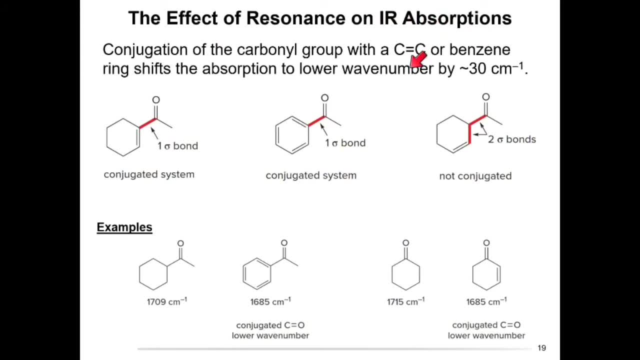 Conjugation of the carbonyl group with a carbon-carbon double bond or benzene ring shifts the absorption to a lower wavenumber. So what is a conjugated system If you have a carbonyl group or, let's say, two double bonds, here separated by a sigma? 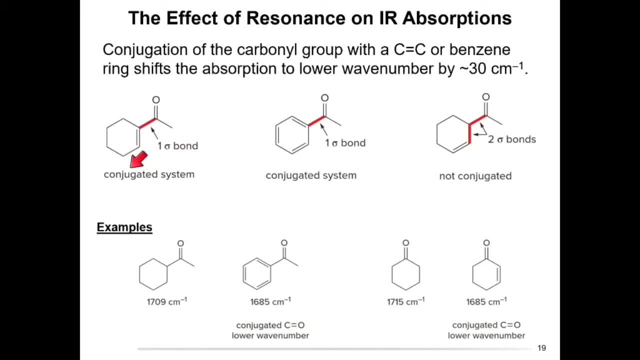 bond. that's considered a conjugated system, And the reason why is because this conjugated system can have resonance, So you can have a single bond here and a double bond here instead. So this is a conjugated system. Over here we also have a conjugated system. 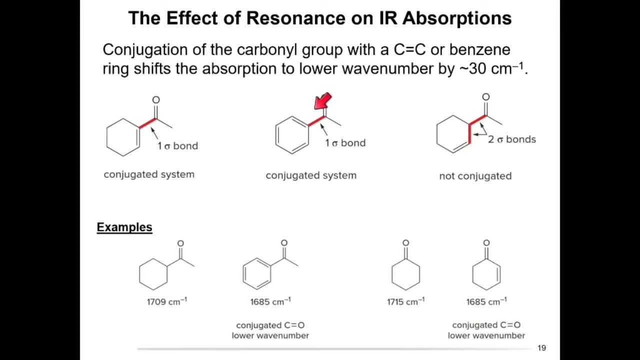 Okay, So we have two double bonds that are separated by a sigma bond, So you can have resonance around this region. The third example here is not considered a conjugated system, And the reason why is because you have two sigma bonds separating the two double bonds. 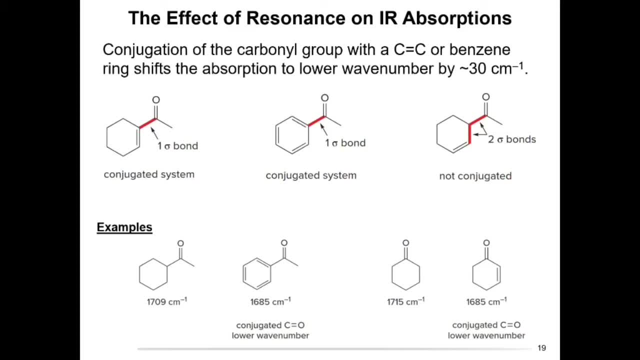 So here's a few examples of when resonance can affect and lower the wavenumber of a specific absorption. So here we have a carbonyl group That's not part of a conjugated system And this absorbs at about 1700 in wavenumber. 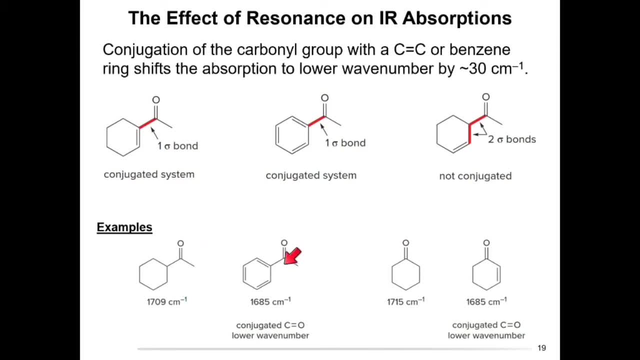 And here we have a carbonyl group that's part of a conjugated system, And so you can see that the absorption occurs at about 1685 wavenumber. So it lowers the absorption of a carbonyl group by about 30 wavenumber. 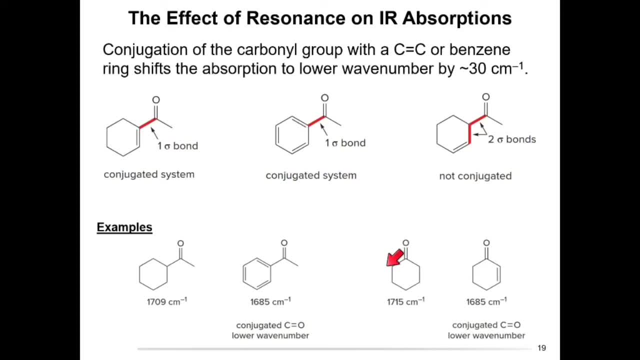 Here's another example. We have a cyclic ring here, So this carbonyl group is a cyclic ring. Okay, So the carbonyl absorbs at about 1715 wavenumber And in a conjugated system the carbonyl absorbs at a lower wavenumber, which is 1685.. 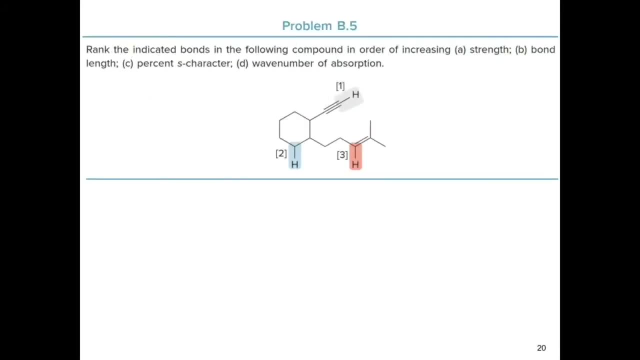 And here's practice. problem number five Rank the indicated bonds in the following compound in order of increasing strength: bond length, percent S, character and wavenumber of absorption. So in this molecule you can see that we're comparing different types of carbon to hydrogen bonds. 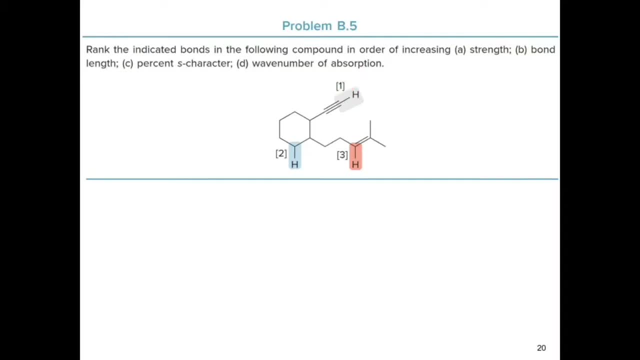 We have this one right here. This one right here is an SP- hybridized carbon to hydrogen bond. The second one here is an SP3- hybridized carbon to hydrogen bond. And then the third one is an SP2- hybridized carbon to hydrogen bond. 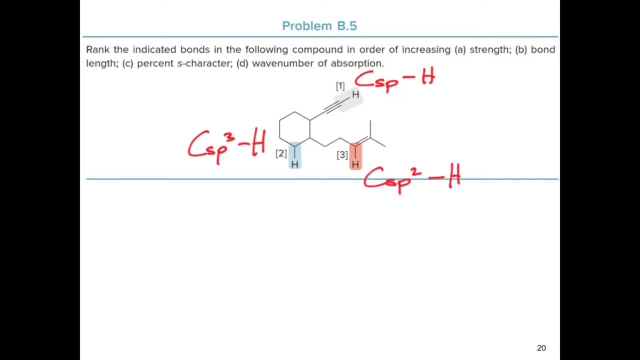 And so, in terms of strength, the SP- hybridized carbon to hydrogen bond- would be the strongest, followed by the SP2- hybridized carbon to hydrogen bond, And then the SP3- hybridized carbon to hydrogen bond. So, in terms of increasing strength, number two here is the weakest, followed by number three. 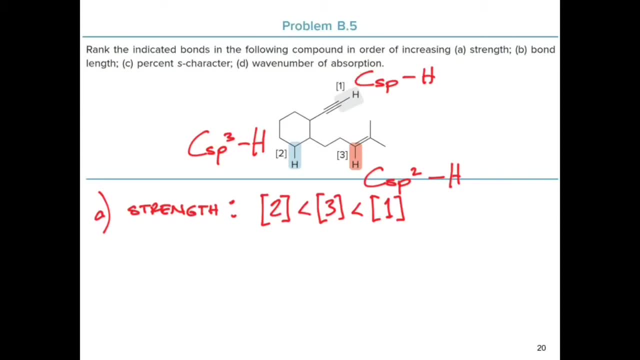 And then the strongest is the first one here, And in terms of percent S character and wavenumber, you can see that strength is actually directly related to the percent S character, And so in terms of increasing percent S character and increasing wavenumber, it would be similar to the strength as shown here. 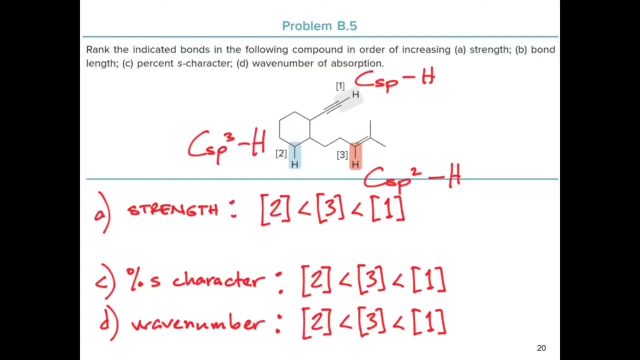 All right. And B, which is bond length. you know that bond length is the opposite of strength, of bond strength, And so it would be the reverse of this. So one is the shortest. So an SP. hybridized carbon to hydrogen bond. 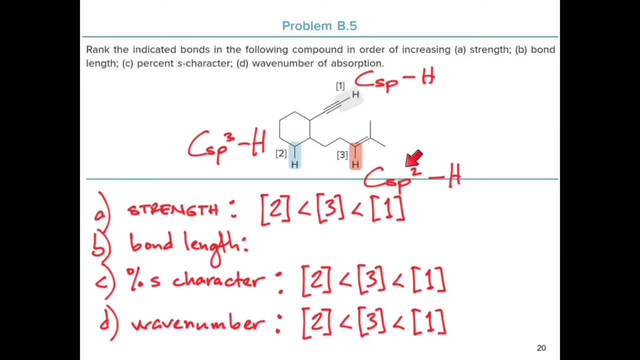 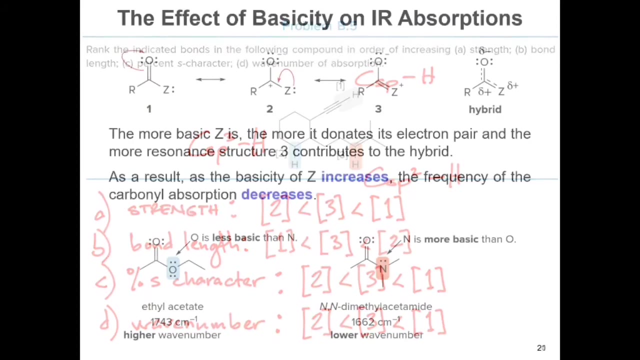 So an SP- hybridized carbon to hydrogen bond, is the shortest, followed by SP2, hybridized carbon to hydrogen bond, And then the longest is an SP3, hybridized carbon to hydrogen bond. as shown here, Passicity can also affect the absorption of infrared. 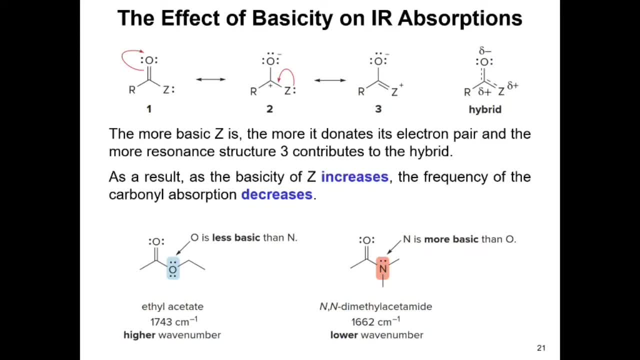 The more basic the atom is, the more it donates its electron pair and the more it contributes to the resonance hybrid. So any functional group that's bonded to a basic atom results in the decrease in its IR absorption. So here we have an ethyl acetate which contains a carbonyl group that's bonded to an oxygen atom. 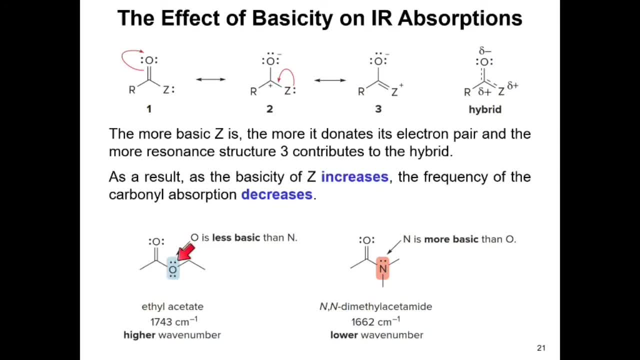 And this oxygen atom is considered basic. So here you can see that the carbonyl group absorbs at about 1743 wavenumber. Over here on the right we have an N-endymethylacetamide which also contains a carbonyl group. 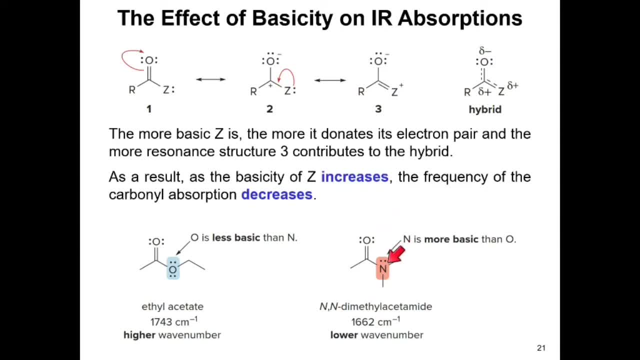 But it's bonded to a more basic atom, which is nitrogen. So since nitrogen is more basic than oxygen, an N-endymethylacetamide will have an absorption lower than ethyl acetate's absorption, which is 1662.. And again, the reason why is because this nitrogen atom contributes more to the resonance hybrid. 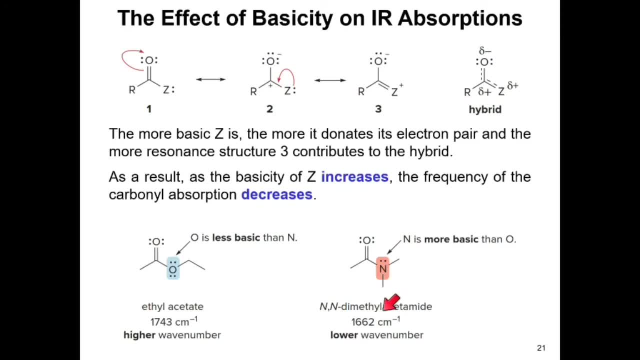 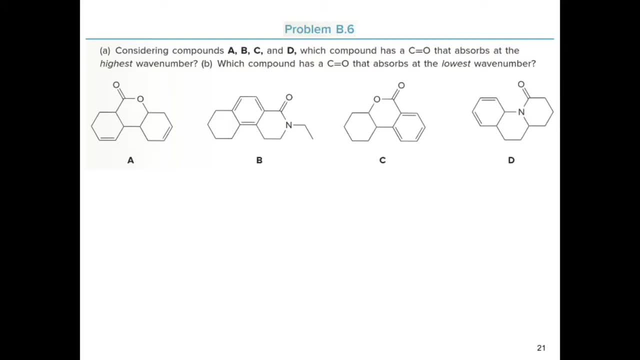 And therefore decreases the absorption of the carbonyl group And therefore decreases the absorption of the carbonyl group. So here's practice problem number six: Considering compounds A, B, C and D: which compound has a carbonyl group that absorbs at the highest wavenumber? 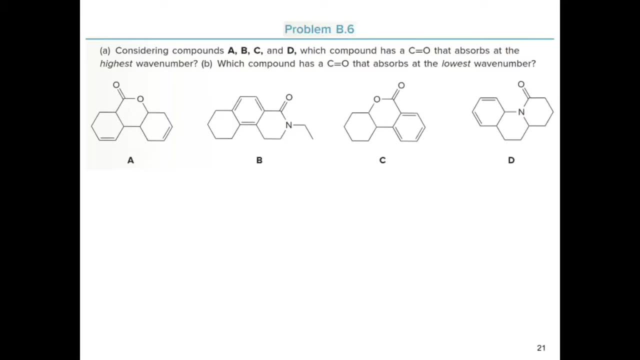 And for part B, which compound has a carbonyl group that absorbs at the lowest wavenumber. So the first thing that I would want to do here is to locate where the carbonyl group is And then figure out which compounds or which atoms are bonded to that carbonyl group. 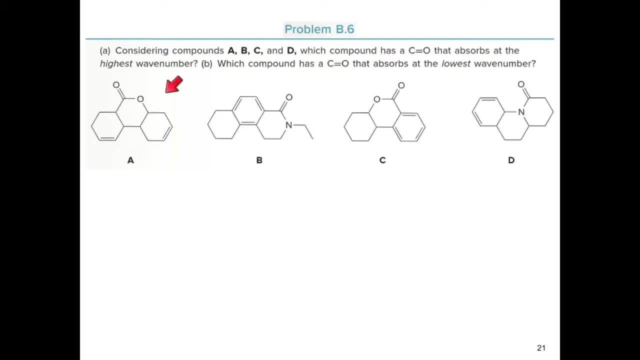 And so for compound A. here you can see that the carbonyl group is bonded to the oxygen atom. And so for compound A. here you can see that the carbonyl group is bonded to the oxygen atom, That's bonded to the carbonyl group. 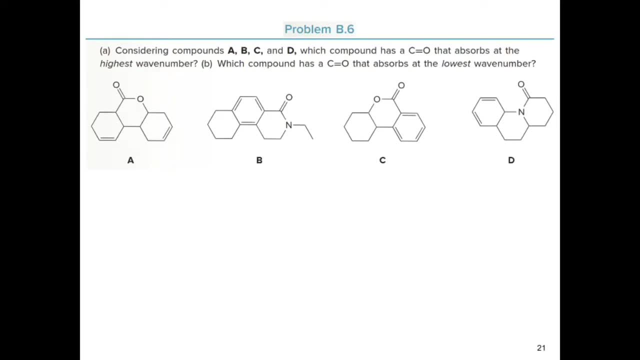 And so we have a basic oxygen atom here. And for compound B, here you can see that we have a carbonyl group that's bonded to a nitrogen atom, And nitrogen is also considered basic because it contains lone pairs of electrons. And when you look at the carbonyl group, it's also bonded next to a double bond. 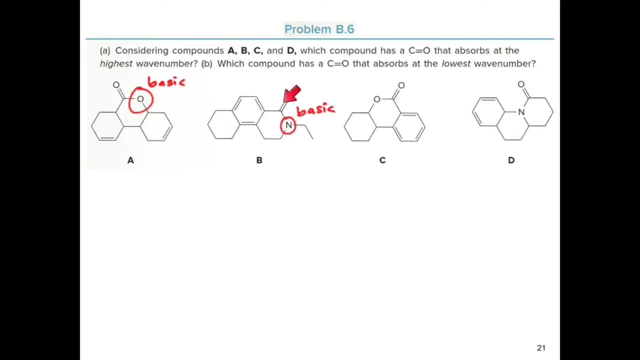 And these two double bonds are separated by a sigma bond, And so what we have here is a conjugated system. And for the third molecule, here you can see that we have a carbonyl group that's bonded to an oxygen atom, which is considered basic. 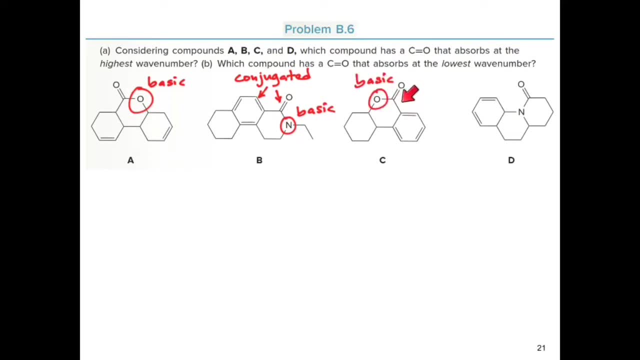 And you can see that we also have a conjugated system here. We have a double bond, two double bonds here, separated by a sigma bond, And for the last molecule you can see that we have a carbonyl group that's bonded to a nitrogen atom. 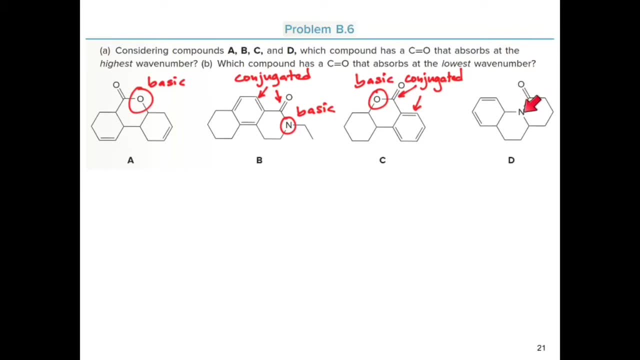 And you can see that we have a carbonyl group that's bonded to a nitrogen atom, which is considered a basic atom. Alright, so now to decide which one would have the highest wavenumber. we would compare the presence of basic atoms and also the presence of conjugated systems. 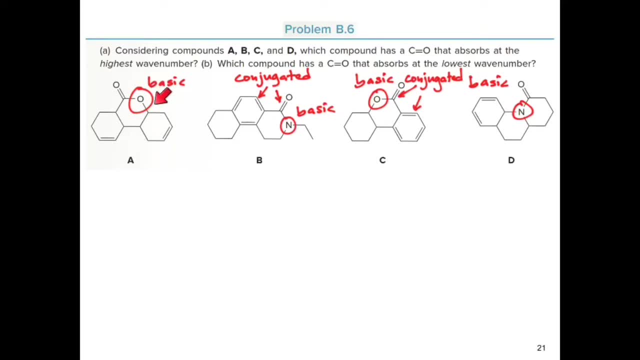 Alright, and so for molecule A, you can see that we only have a basic atom And it doesn't contain any conjugated systems. We only have a conjugation here, And if we compare molecule A with molecule D, you can see that nitrogen is the more basic atom. 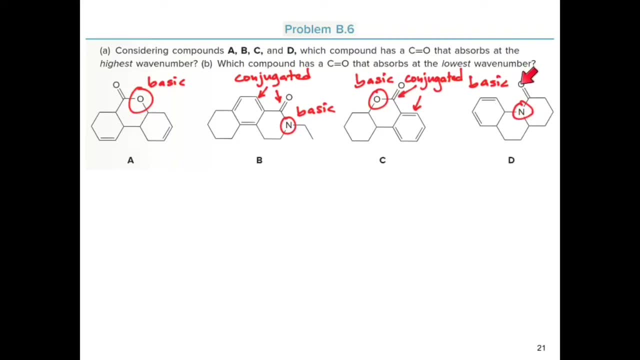 And so the wavenumber here for the carbonyl group would be lower compared to molecule A, And so molecule A then in this case would have the highest wavenumber, Because you know that a conjugated system would have an even lower wavenumber. 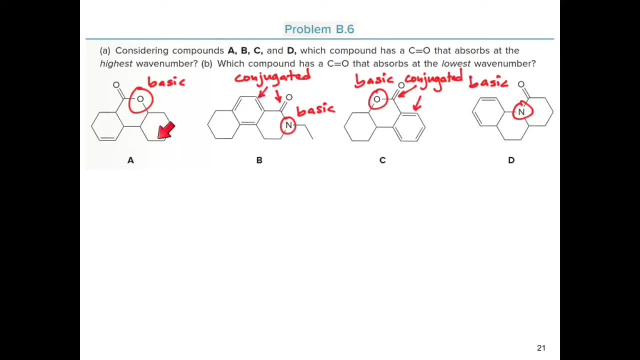 For the carbonyl group, And so again, molecule A would have the highest wavenumber And the molecule with the lowest wavenumber would be the molecule containing a conjugated system and the more basic atom that's bonded to the carbonyl group. 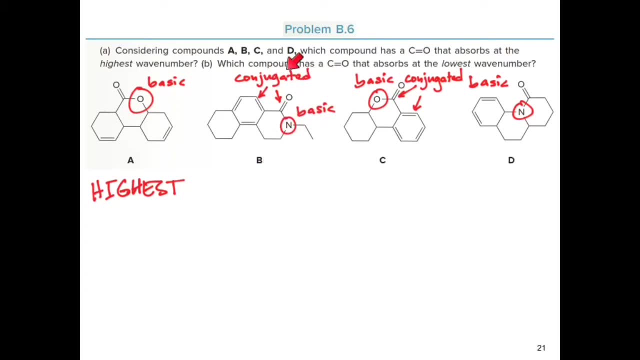 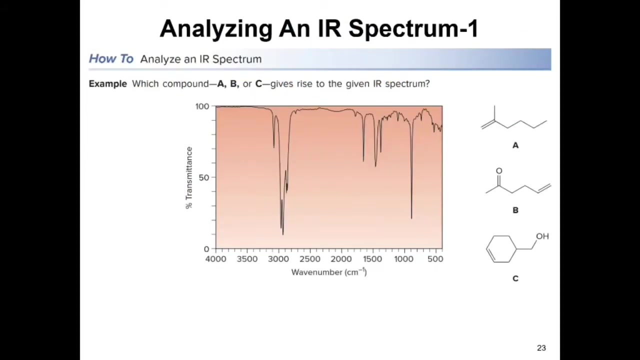 So you can see here that we have molecule B containing a conjugated system and a more basic nitrogen atom, And so therefore molecule B would have the lowest wavenumber. So how do we analyze an IR spectrum? Here's an example: Which compound- A, B or C- gives rise to the given IR spectrum. 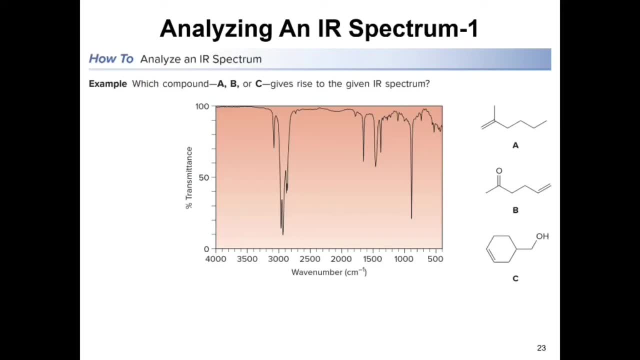 So whenever you're analyzing an IR spectrum, the best approach here is to divide the IR spectrum into four different regions. So we have the fingerprint region, which occurs between 400 and 1500 wavenumber. We have the double bond region. 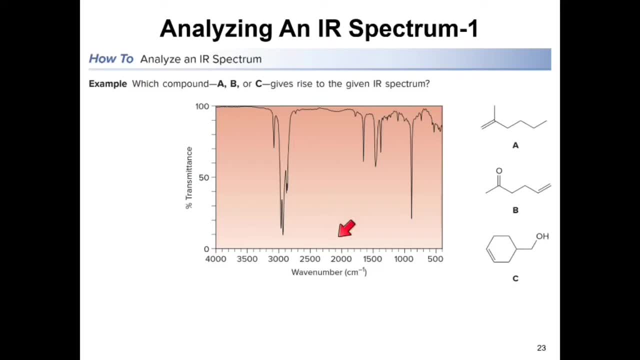 which occurs between 1500 and 200 wavenumber. And then we have the triple bond region, which occurs between 2000 and 2500.. And then anything above 2500 is the single bond region involving hydrogen atoms. All right, 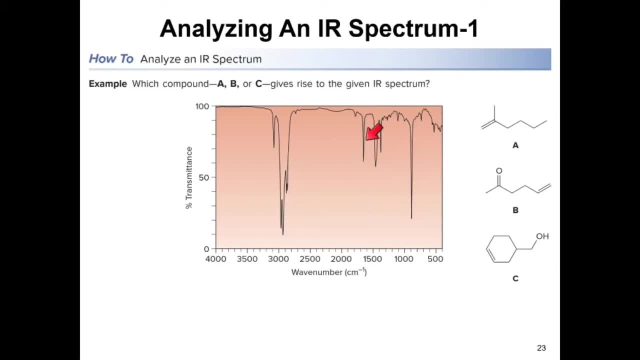 And so you can see that we have. So here we can focus on the functional group region, which is between 1500 and 4000 wavenumber, And so you can see that we have several peaks here. We have this one over here. 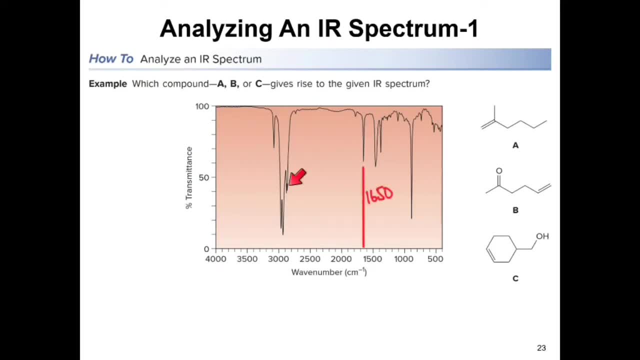 which occurs at about 1650 wavenumber. We have these peaks over here as well, between 2800 and 3000 wavenumber, And then the last one right up here, which occurs at about 3100 wavenumber. 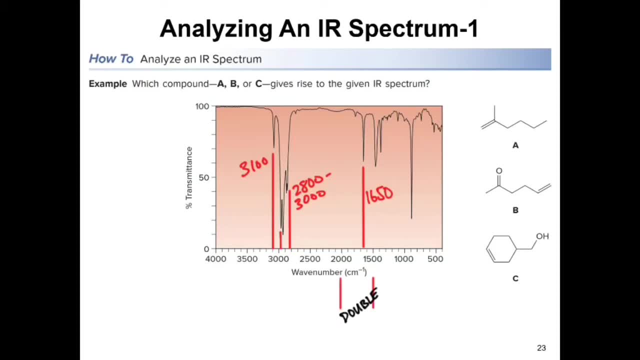 All right, And so again we divide the IR spectrum into four different regions. So we have the double bond here, and the 1650 wavenumber most likely corresponds to a carbon-carbon double bond, And then in the triple bond region, 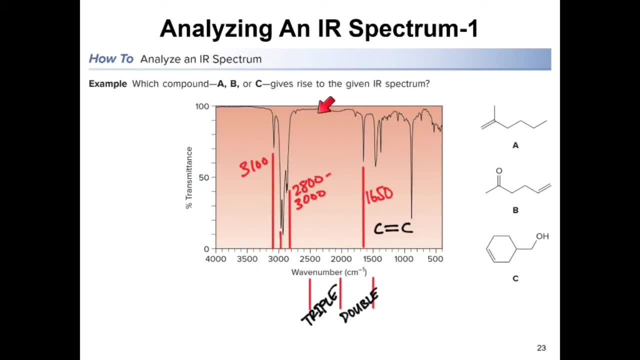 you can see that we don't really have any prominent peaks here, And so there must not be any carbon-carbon triple bond, And over here we have the single bond to hydrogen region, And so you can see that it occurs between 2500 and about 3500. 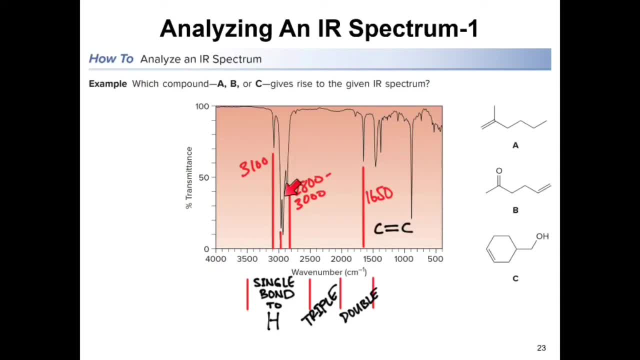 So these peaks right here must correspond to a carbon-to-hydrogen single bond, And when you look at the table, you can see that between 2800 and 3000,. what you have here is an sp3 hybridized carbon-to-hydrogen bond. 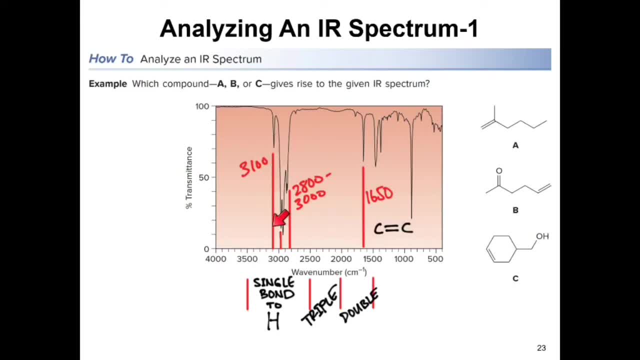 All right. And then at 3100, we have an sp2- hybridized carbon-to-hydrogen bonds- And so most likely we have molecule A here, because when you look at molecule A, it contains a bunch of carbon-to-hydrogen bonds. 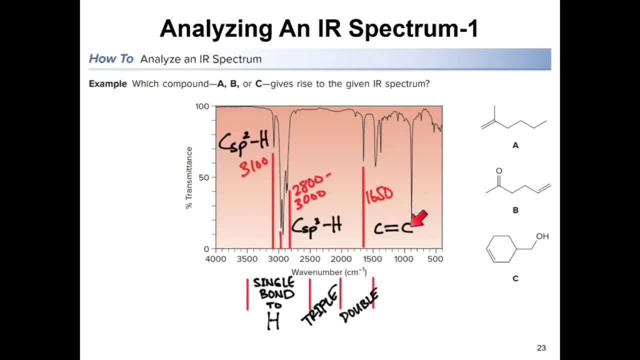 as well as carbon-to-carbon double bond, And so the carbon-carbon double bond has a peak at 1650.. And then you have an sp2- hybridized carbon-to-hydrogen bond Here, which occurs at 3100.. 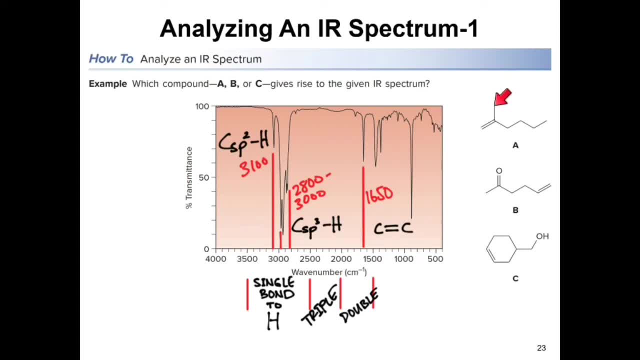 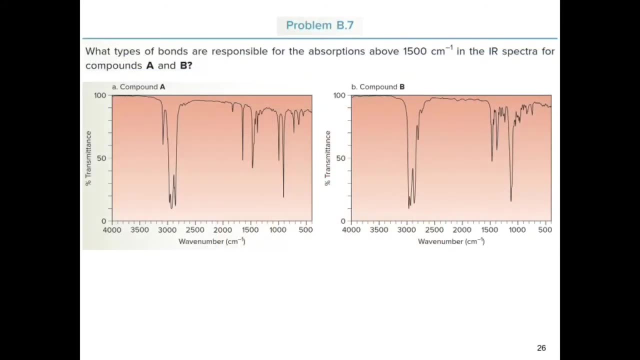 And finally you have a bunch of sp3, hybridized carbon-to-hydrogen bonds, which occur at about between 2800 and 3000 wave number. So we have molecule A. So here's practice problem number seven: What types of bonds are responsible? 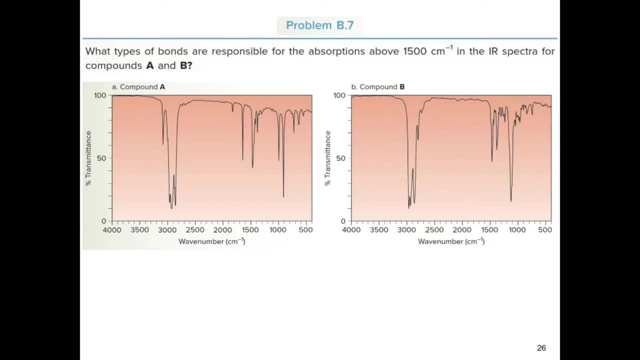 for the absorptions above 1500 wave number in the IR spectra for compounds A and B. So if you're already familiar with the different types of bonds, different regions of the IR spectrum, then you can go ahead and identify the different peaks. 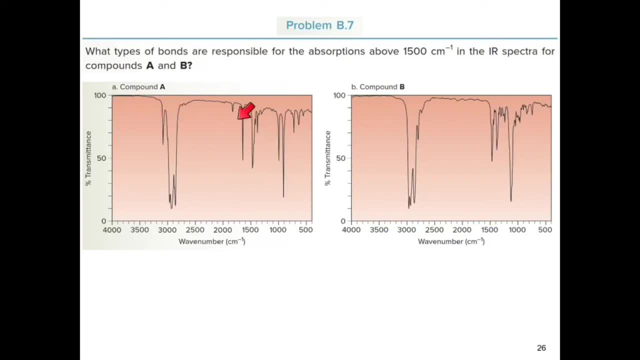 So above 1500, we have these peaks right over here, So we have a peak around 1650.. We have several different peaks between 2800 and 3000 wave number and another peak at about 3100.. And so the 1650 wave number. 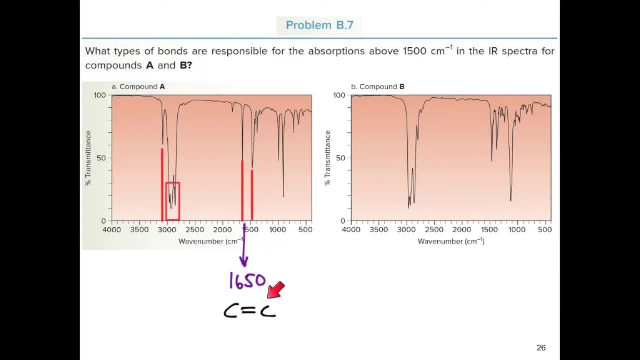 the peak here at 1650, corresponds to a carbon-carbon double bond, And over here, between 2800 and 3000 wave number, these peaks correspond to a carbon-to-hydrogen bond, more specifically sp3, hybridized carbon-to-hydrogen bond. 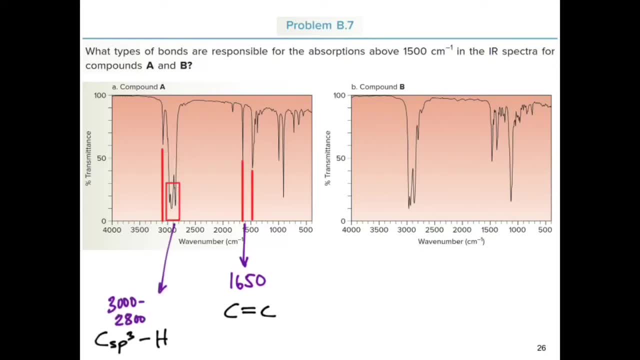 And the last peak here, around 3100, corresponds to another carbon-to-hydrogen bond, but more specifically sp2, hybridized carbon-to-hydrogen bond. So according to this IR spectrum, these are the three types of bonds that are present in compound A. 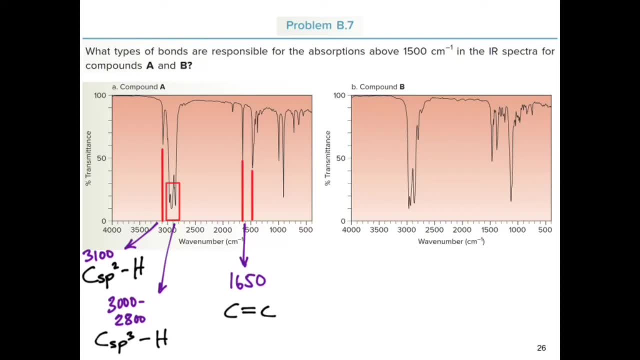 And for the second compound. here we'll do the same thing. So we're going to identify the characteristic peaks that are present above 1500.. And so the only peaks that are present are these ones right here, And so we have several different peaks. 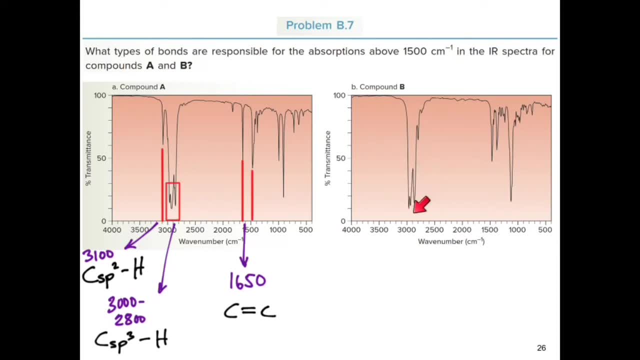 that occur between 2800 and 3000 wave number, And so these peaks correspond to the sp3 hybridized carbon-to-hydrogen bond, And so this is the only type of bond that's present in this compound. In the next couple of slides, 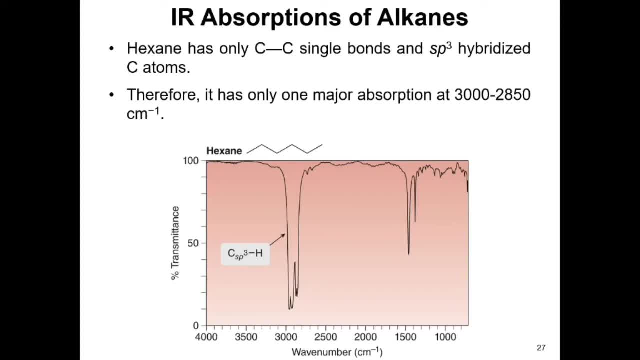 we're going to take a look at the infrared absorptions of different types of organic compounds, such as alkanes, alkenes, alkynes, alcohols and so on and so forth, containing different types of functional groups. So the first one here is the IR absorption. 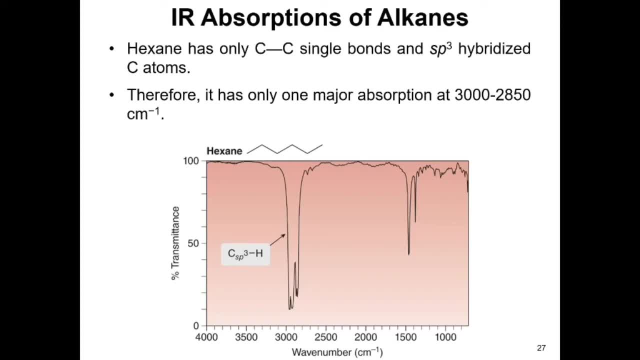 or IR spectrum of hexane, which is a type of an alkane. And you know that alkanes only contain one single type of bond, and that's the sp3, hybridized carbon-to-hydrogen bond, And so they have a major absorption. 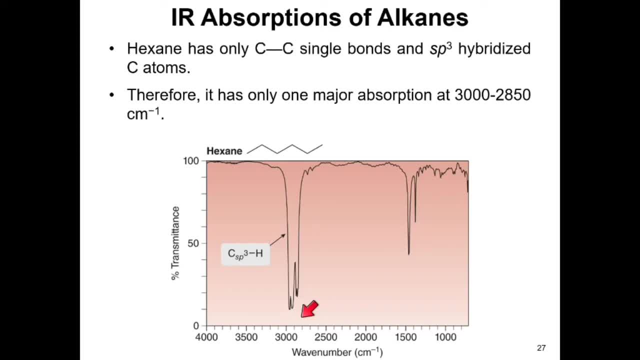 between 3000 and 2800 wave number, And so you have several different peaks here. that ranges between 2800 and 3000 wave number, And again these peaks correspond to the sp3, hybridized carbon-to-hydrogen bond. 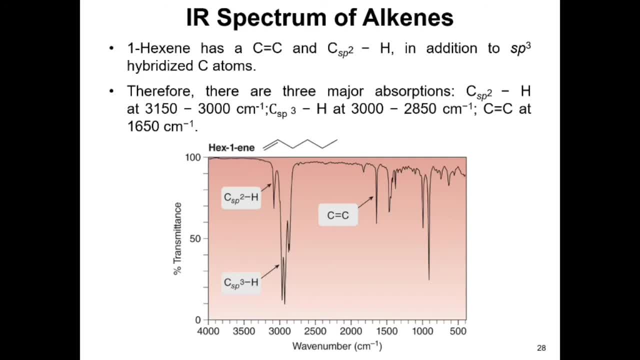 Shown here is the IR spectrum of hexane, which is an example of an alkene. So when you look at the chemical structure of this alkene, you can see that it contains several different types of bonds. It contains a carbon-carbon double bond. 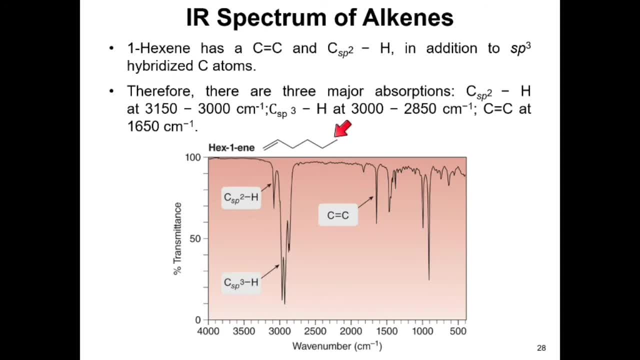 It contains two different types of carbon-to-hydrogen bonds. You have the sp3 hybridized carbon-to-hydrogen bond and also sp2 hybridized carbon-to-hydrogen bond. So theoretically you should have three major absorptions In an alkene's IR spectrum. 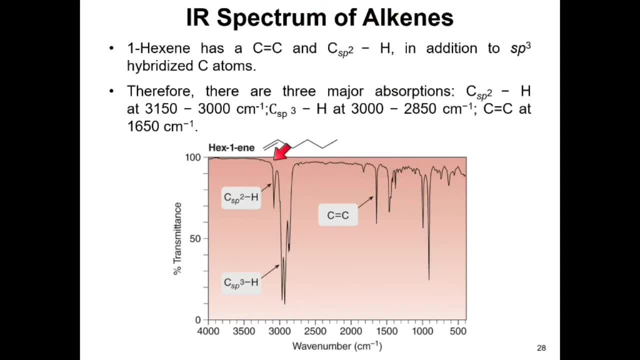 So shown here, we have one, two and three different major absorptions. So we have the carbon-to-carbon double bond, which occurs at 1650 wave number. We have the sp3, hybridized carbon-to-hydrogen bonds. 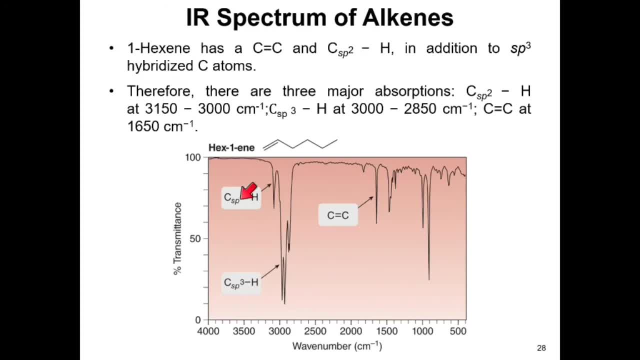 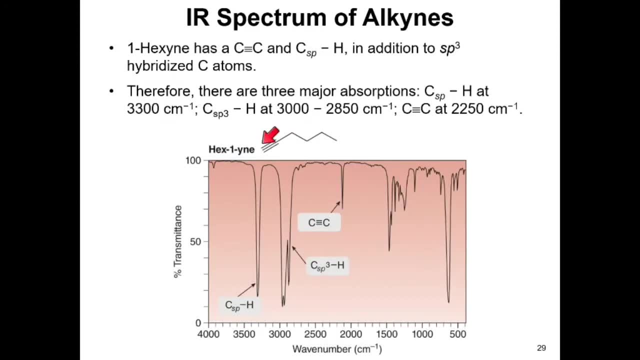 which occur between 2800 and 3000 wave number, And finally, sp2, hybridized carbon-to-hydrogen bond, which occurs around 3100.. So this is what an IR spectrum of an alkyne looks like. So what we have here is the IR spectrum for Hex-1-Ine. 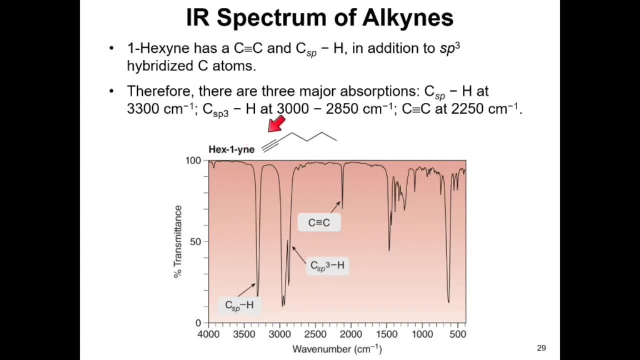 And so when you look at the chemical structure of alkynes, you can see that there are three different bonds. You have a carbon-carbon triple bond. You have two different types of carbon-to-hydrogen bonds. You have the sp3 hybridized carbon-to-hydrogen bond. 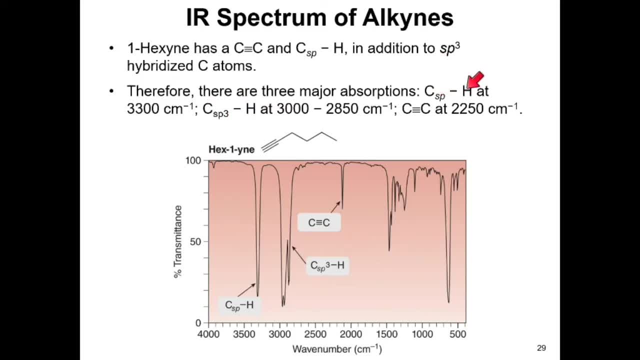 as well as an sp, hybridized carbon-to-hydrogen bond, And so you would expect three major absorptions in its IR spectrum. So here you can see that there's a peak at about 2200, which corresponds to a carbon-carbon triple bond. 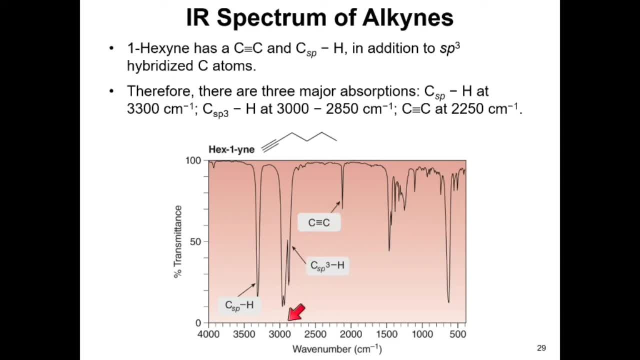 And then you also have several peaks between 2800 and 3000 wave number, which correspond to sp3- hybridized carbon-to-hydrogen bonds. And finally we have a peak at about 3300 wave number, which corresponds to an sp- hybridized carbon-to-hydrogen bond. 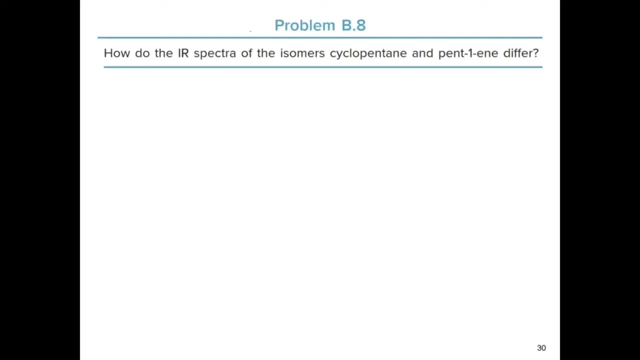 So here sparks problem number eight: How do the IR spectra of the isomer cyclopent and pent-1-ene differ? So here we have two different types of organic compounds. We have cyclopentane and pent-1-ene. 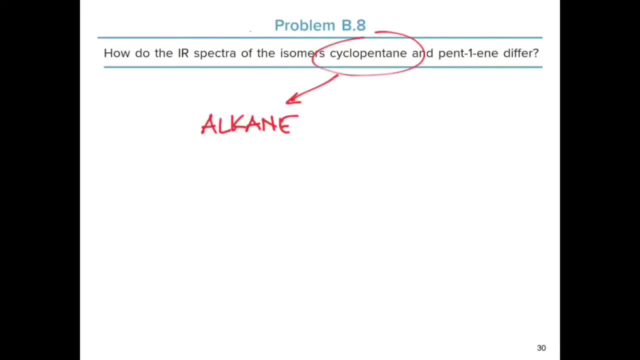 Cyclopentane is an example of an alkane and pent-1-ene is an example of an alkene, And so you learned in the previous slides that alkanes typically have one major absorption, and that occurs between 2800 and 3000 wave number. 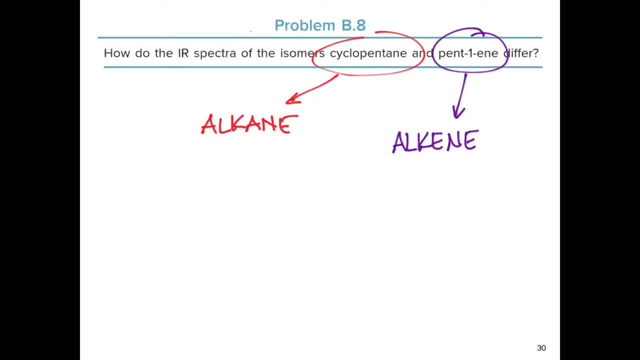 And that absorption corresponds to sp3, hybridized carbon-to-hydrogen bond. In alkanes we have three major absorptions. One occurs at between 2800 and 3000 wave number, which is also the absorption for sp3- hybridized carbon-to-hydrogen bonds. 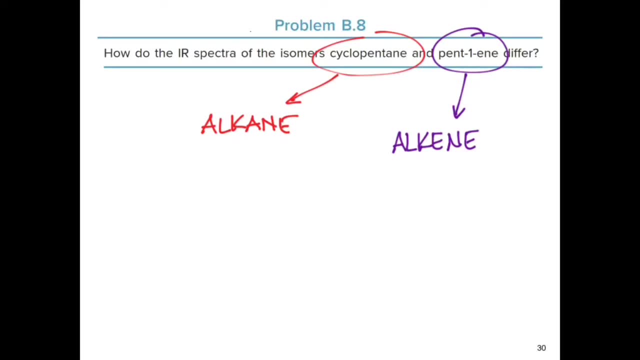 And then the two other absorptions are for the carbon-carbon double bond and also sp2, hybridized carbon-to-hydrogen bond, And so the carbon-carbon double bond occurs at 1650 wave number, whereas the sp2 hybridized carbon-to-hydrogen bonds. 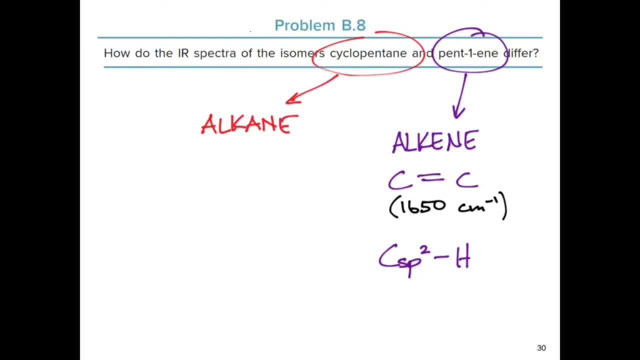 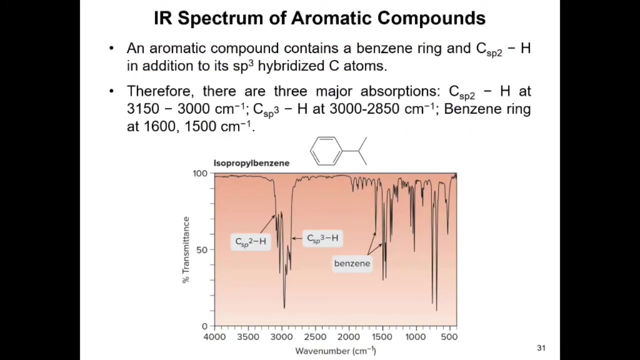 occur at about 3100 wave number, And so alkanes will have two additional absorptions or peaks, one at 1650 and the other one at 3100 wave numbers. Aromatic compounds are compounds containing a benzene ring, So that means that they're going to have two different types of carbon-to-hydrogen bonds. 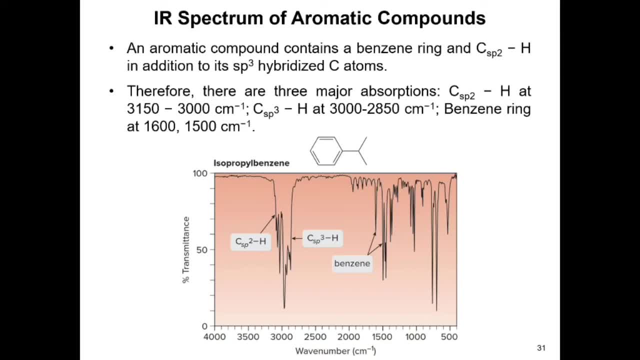 There's the sp2 hybridized carbon-to-hydrogen bond and sp3 hybridized carbon-to-hydrogen bonds, And so aromatic compounds typically have three major absorptions: One between 3100 and 3000 wave number, which is this one right here? 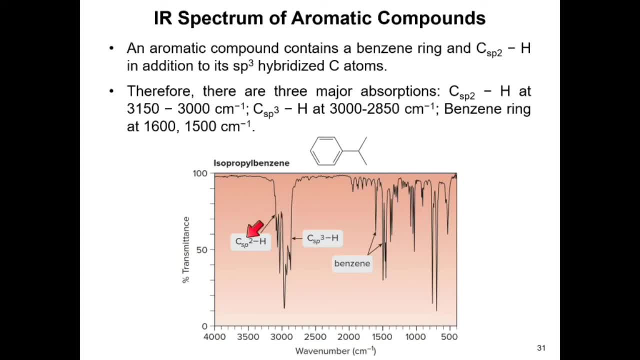 And this corresponds to the sp2 hybridized carbon-to-hydrogen bond. We also have absorptions between 2800 and 3000 wave number, And this absorption corresponds to the sp3 hybridized carbon-to-hydrogen bond. And finally, we have the benzene absorption. 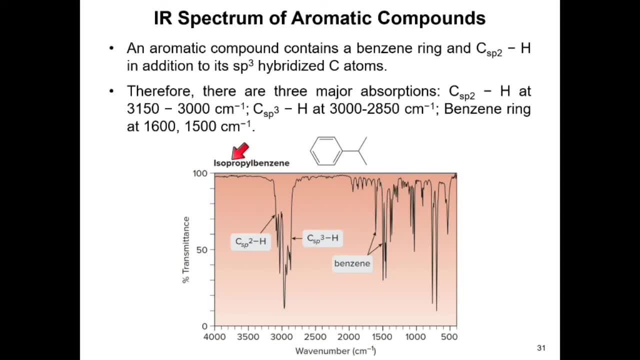 which occurs at two different wave numbers, one at 1600, right over here, and the other one at 1500.. So again, these two peaks correspond to the benzene ring Shown here is the IR spectrum of butan-2-ol. 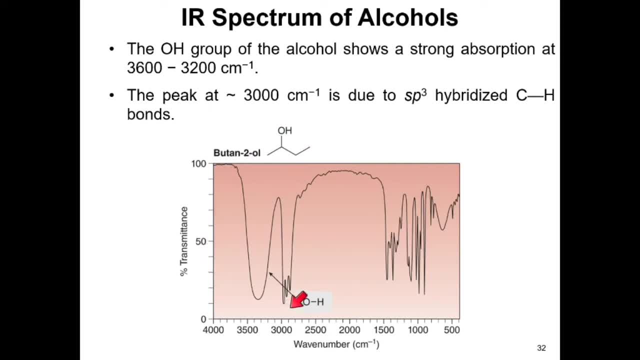 So you can see here that alcohols typically have a broad strong absorption between 3200 and 3600. And this absorption corresponds to the hydroxy group coming from the alcohol. And alcohols also have absorptions between 2800 and 3000 wave number. 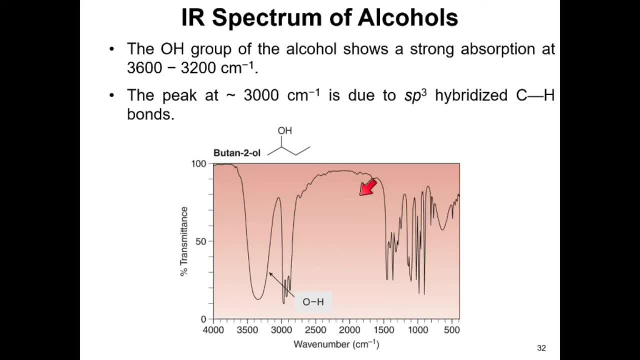 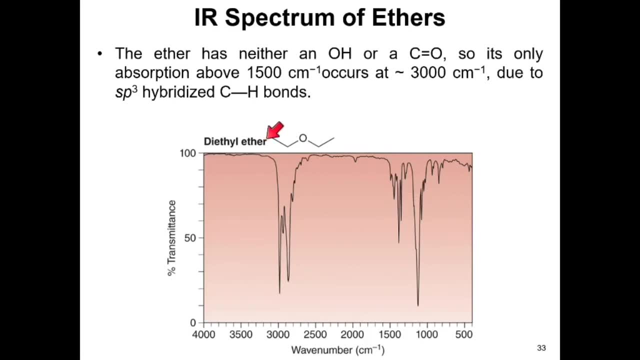 And these absorptions correspond to sp3, hybridized carbon-to-hydrogen bonds. And here we have the IR spectrum of diethyl ether And, as you can see, based on its chemical structure, you can see that ethers don't have any hydroxy group. 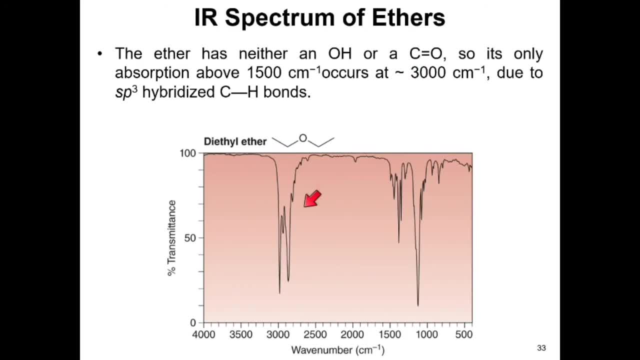 or a carbonyl group, And so the only absorption that occurs in the IR spectrum above 1500 is between 2800 and 3000 wave number, And these absorptions correspond to the sp3- hybridized carbon-to-hydrogen bonds. 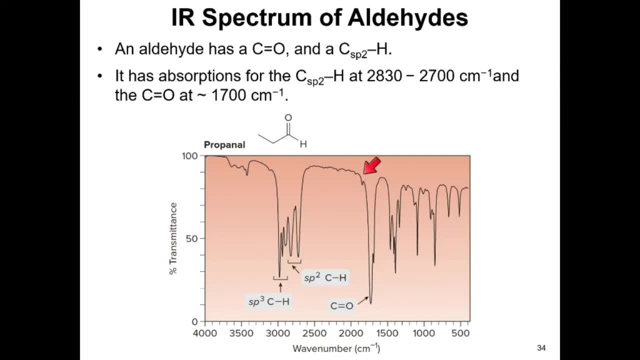 And this is what the IR spectrum of aldehydes look like. So what we have here is the IR spectrum for this compound, propanal. So looking at the structure of this compound, you can see that it has a carbonyl group. 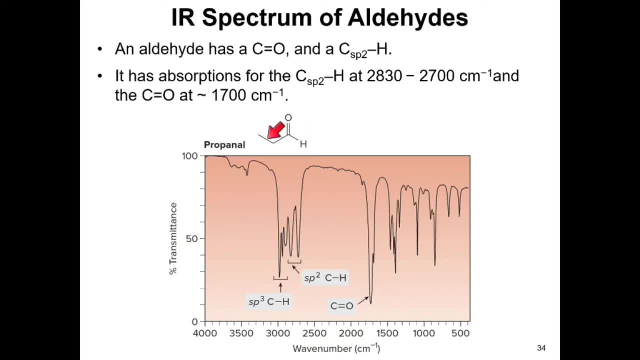 it has an sp2 hybridized carbon-to-hydrogen bond as well as sp3 hybridized carbon-to-hydrogen bonds, And so you would expect three major peaks for aldehydes above 1500 wave number. So the first one here occurs at about 1700 wave number. 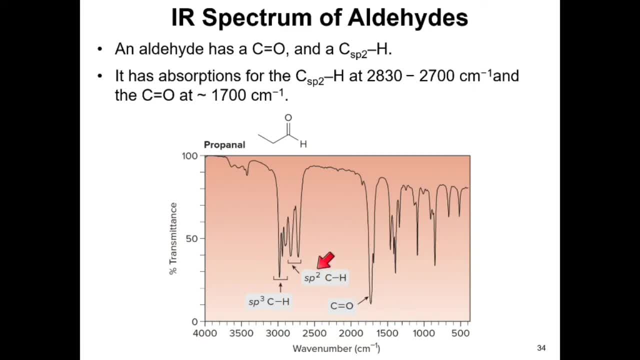 which corresponds to the carbonyl group. And then we also have two different types of carbon-to-hydrogen bonds here. The sp2 hybridized carbon-to-hydrogen bond occurs between 2800 and 2700 wave number, And for the sp3 hybridized carbon-to-hydrogen bond, 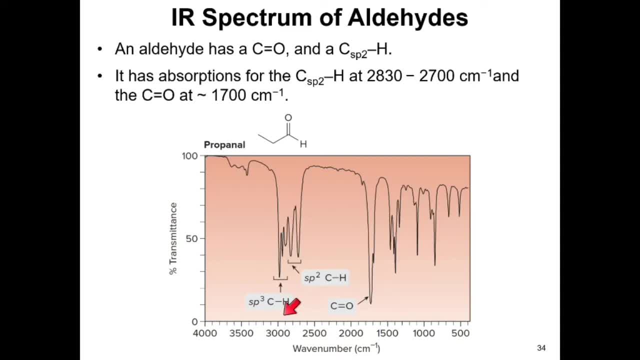 occurring at about 3000 wave number. So you can see that these absorptions here for the carbon-to-hydrogen bonds decreased And this is due to the presence of the carbonyl group. So sp2- hybridized carbon-to-hydrogen bonds- typically occur above 3000 wave number. 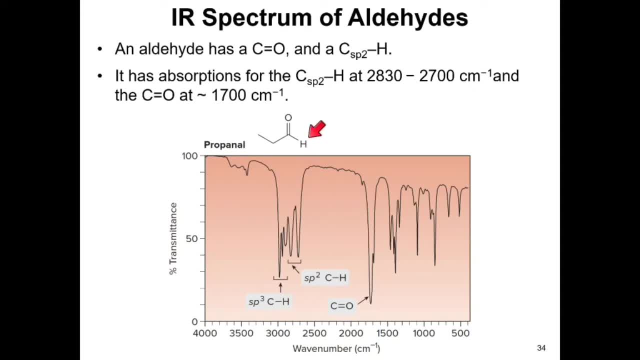 roughly around 3100 wave number. But because this hydrogen is bonded to a carbonyl group, its energy decreases. So again from 3100 to about 2800.. So that's why this sp2, hybridized carbon-to-hydrogen bond. 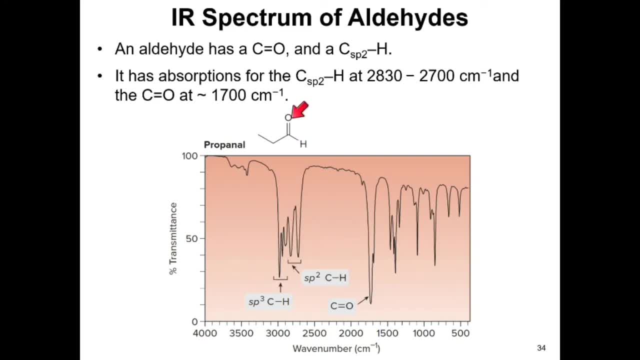 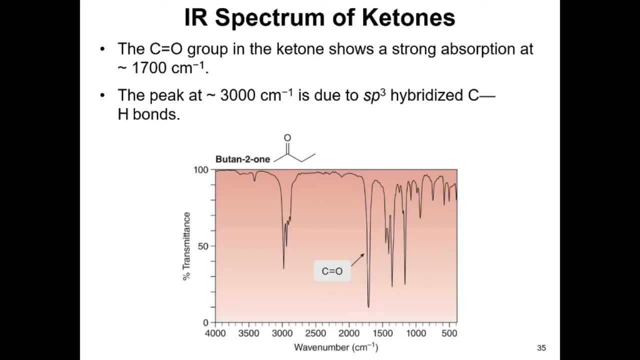 occurs at about 2800.. Again, due to the presence of the carbonyl group, The infrared spectrum of ketones looks a little bit different compared to the IR spectrum of aldehydes, And the reason why is because in ketones the carbonyl group 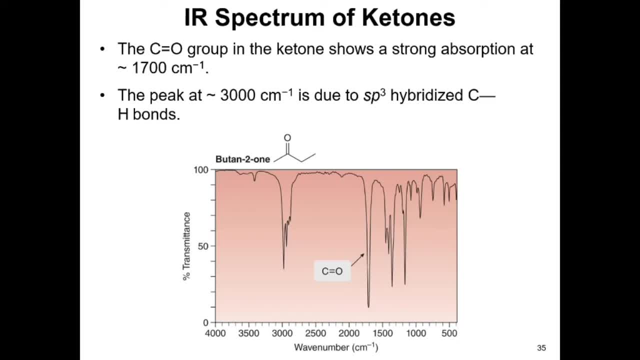 is bonded to two carbon atoms, Whereas in aldehydes the carbonyl group is bonded to one hydrogen and one carbon, And so that means that ketones would have only two different types of absorptions above 1500 wave number, And the carbonyl group would have an absorption around 1700. 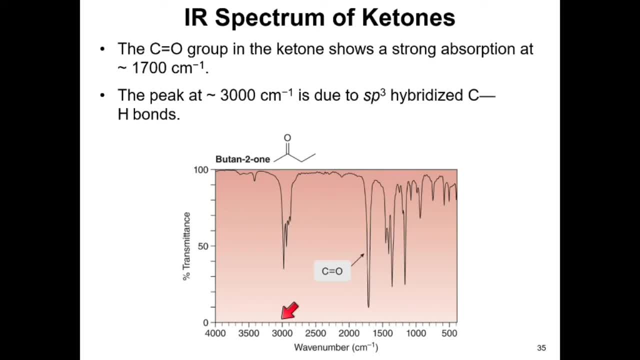 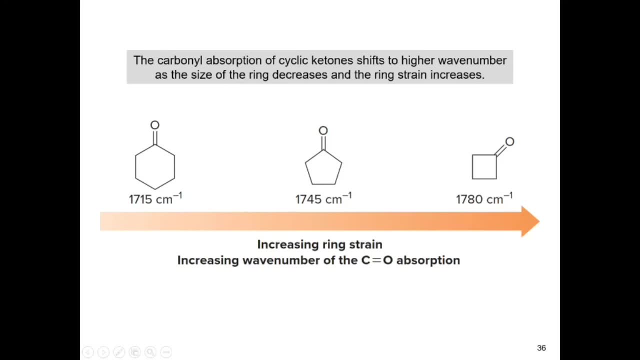 And then sp3, hybridized carbon-to-hydrogen bonds between 2800 and 3000 wave number. The size of the ring can also affect the absorption of the carbonyl group, As the carbonyl group is bonded to a cyclic ring. 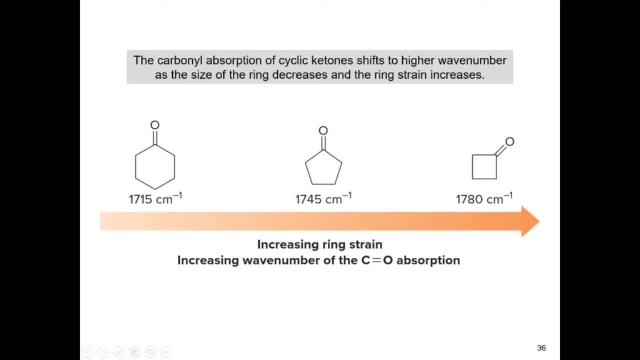 the wave number increases as the size of the ring decreases, And the reason why is because of the ring strain. As the size of the cyclic ring decreases, the ring strain increases And therefore the absorption of the carbonyl group also increases. 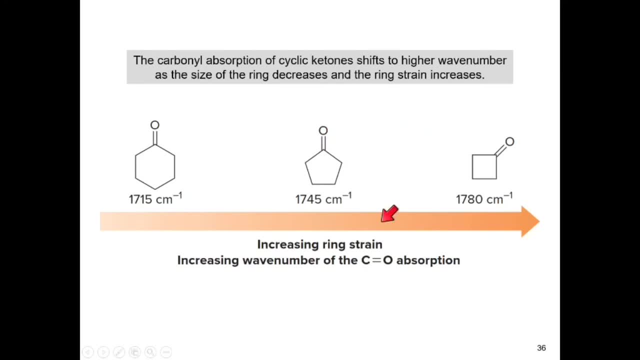 So here you can see that as the size of the cyclic ring decreases, ring strain increases And this also increases the wave number of the carbonyl absorption from 1715 wave number all the way to 1780 wave number. Here's practice problem number nine. 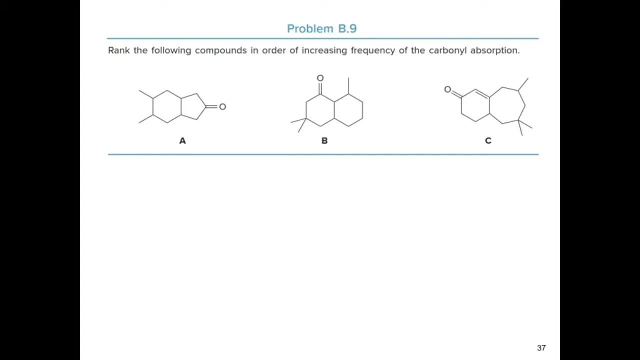 Rank the following compounds in order of increasing frequency of the carbonyl absorption. So the first thing that you should do here is to analyze the carbonyl group. Is it bonded to a six-carbon ring, five-carbon ring or four-carbon ring? 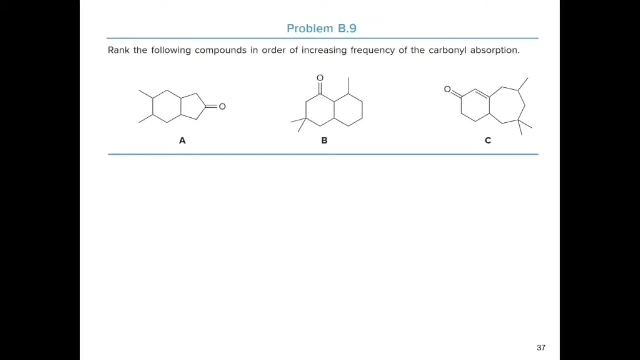 So whenever you look at the first one here, you can see that the carbonyl group is bonded to five carbons, And so we have a five-membered ring. here, The second molecule, we have a carbonyl group that's bonded to six carbon atoms. 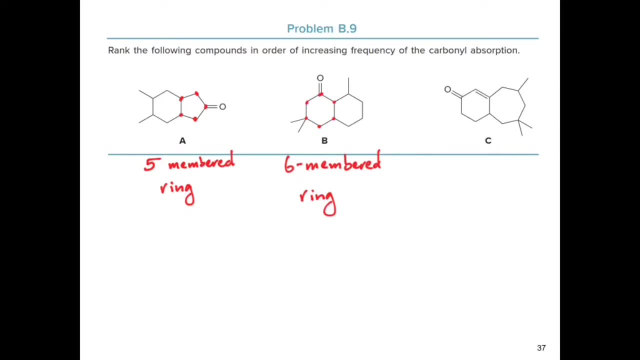 or a cyclic ring that contains six carbon atoms, So we have a six-membered ring here. And then for molecule C we have a carbonyl group that's bonded to a six-membered ring, And so you can see that the lower the number of carbons in a ring, 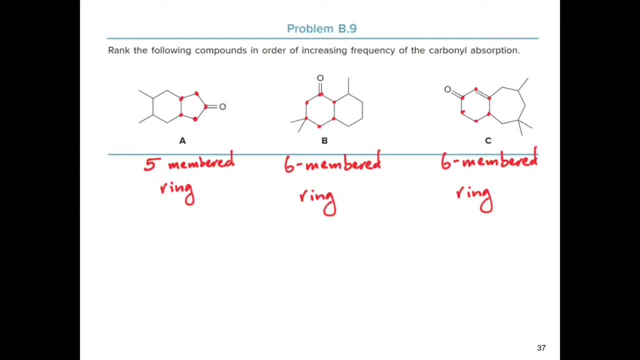 the higher the strain, And so this would actually increase the frequency of the carbonyl absorption, And so A. that means that A has the highest frequency, And if we're comparing molecules B and C here, you can see that molecule C has a conjugation. 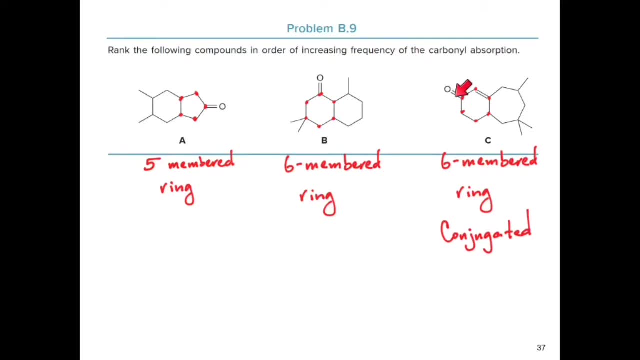 has a conjugated system, So we have two double bonds here that are separated by a sigma bond. So there is some resonance happening here, because it's a conjugated system, And so conjugation will actually decrease the absorption of the carbonyl functional group. 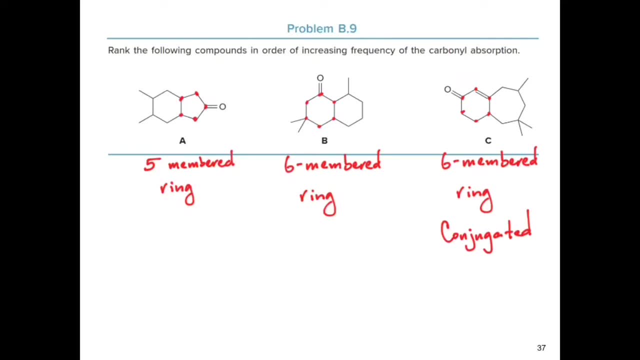 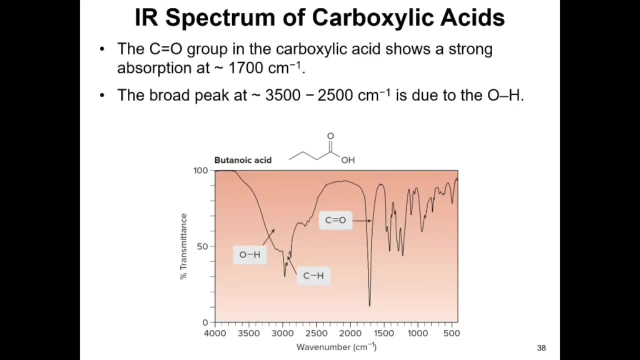 And so therefore, C has the lowest frequency. So again from CBA. So here we have the infrared spectrum of a carboxylic acid, butanoic acid. So here you can see, based on its chemical structure, that it contains several different functional groups. 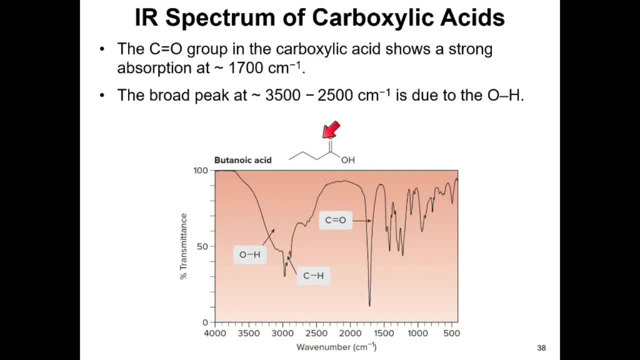 It has a carbonyl group, it has a hydroxy group and it has much of sp3, hybridized carbon-to-hydrogen bonds, And so you would expect a total of three major absorptions above 1500 wavenumber. 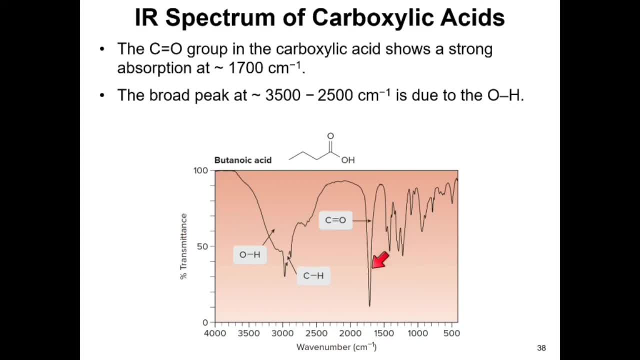 So here we have a carbonyl group that absorbs at about 1700 wavenumber, a hydroxy group, which is a broad absorption, between 3500 and 2500, and as well as sp3, hybridized carbon-to-hydrogen bonds. 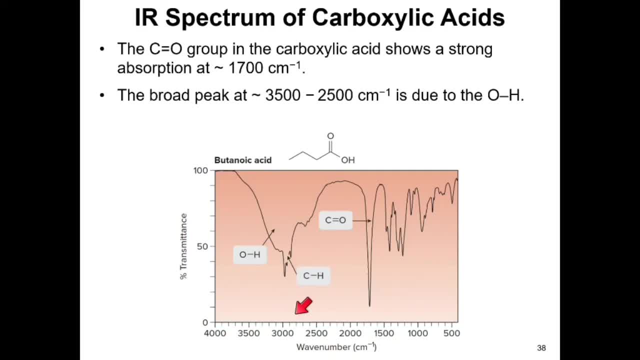 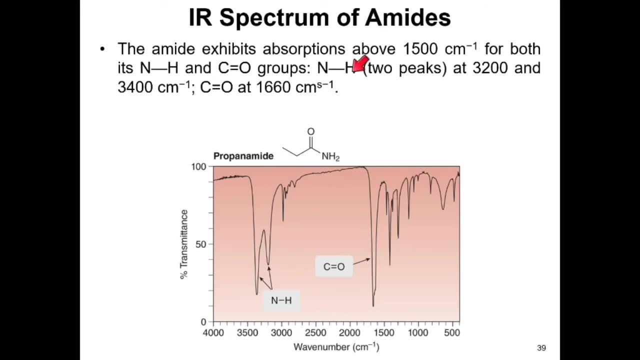 which occur below 3000, between 2800 and 3000 wavenumber. Shown here is the infrared spectrum for propanamide, which is an example of an amide, As you can see here, based on its chemical structure. 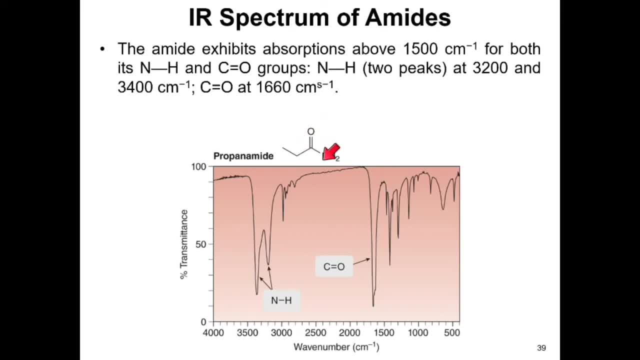 it contains a carbonyl group and an amine group. In addition, propanamide also contains sp3, hybridized carbon-to-hydrogen bonds, And so you would expect a total of three major absorption peaks for this molecule. So here we have the carbonyl group. 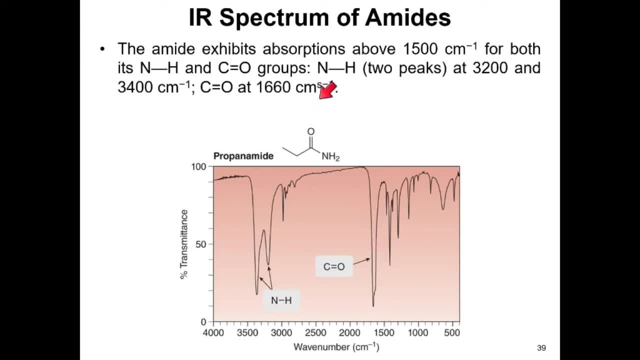 which has an absorption at about 1660 wavenumber. It has two peaks, two absorption peaks for the amine group, which occurs at 3200 and 3400 wavenumber. In addition, the sp3- hybridized carbon-to-hydrogen bonds. 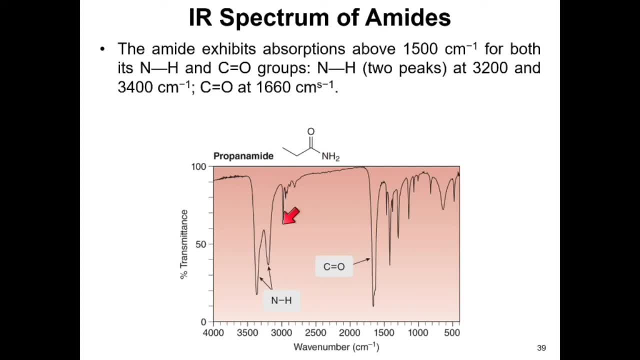 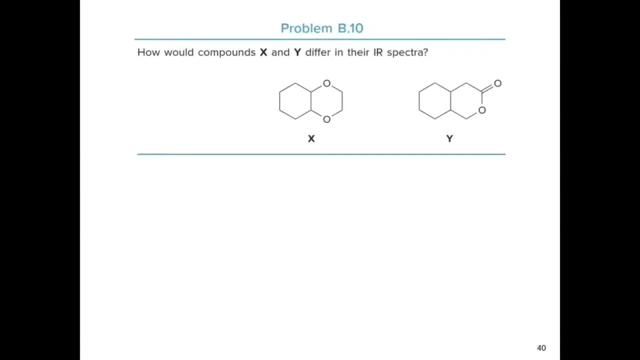 also absorb at about 3000, between 2800 and 3000 wavenumber, as shown here. Here's practice problem number 10. How would compounds X and Y differ in their IR spectra? So when you look at compounds X and Y here, 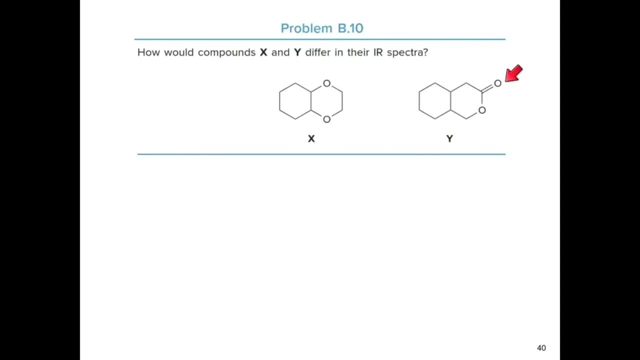 you can see that compound Y contains a carbonyl group, whereas compound X does not contain a carbonyl group, And so you would expect an absorption at about 1700 or 1680 wavenumber for compound Y and no absorption around that region for compound X. 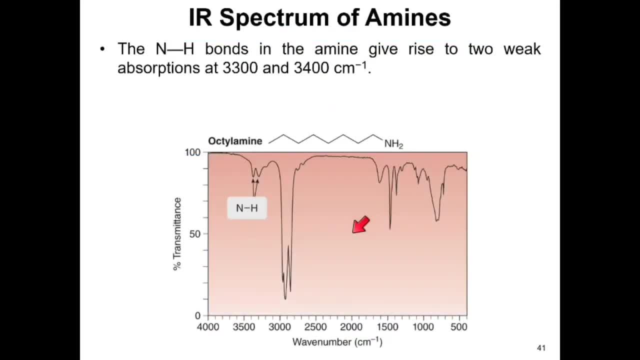 And this is what an IR spectrum for amines look like. So what we have here is the IR spectrum for octylamine, So it contains eight carbon atoms and then an amine group at the end. So you can see that octylamine contains two peaks. 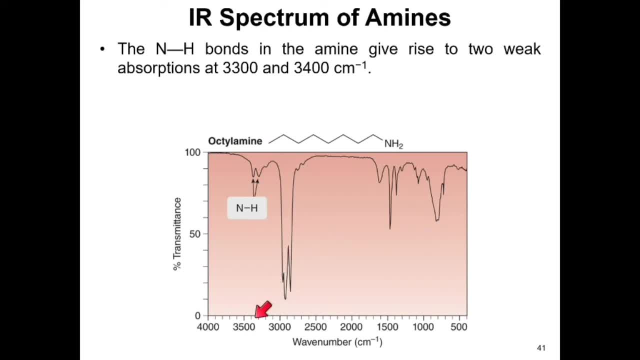 one at 3200 and the other one at 3400 wavenumber. And in addition to these two peaks, octylamine also contains sp3- hybridized carbon-to-hydrogen bonds, as shown here. So you can see that the sp3 hybridized carbon-to-hydrogen bonds- 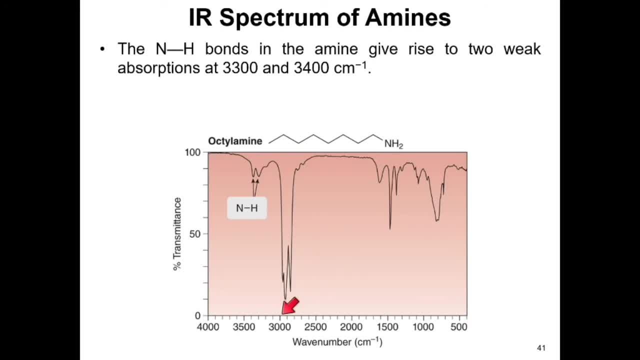 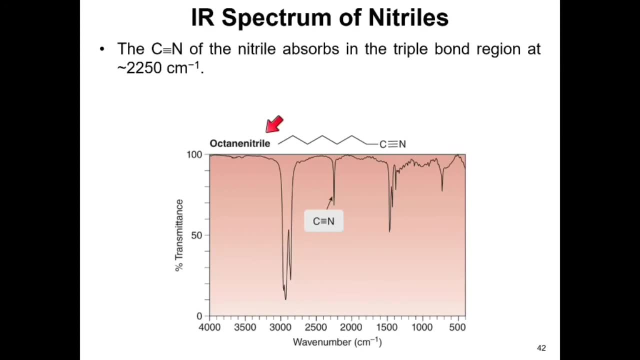 absorb between 2800 and 3000 wavenumber. So nitriles are compounds that contain a carbon-to-nitrogen triple bond. So here we have octane nitrile and this is the IR spectrum for this compound. So you can see that carbon-to-nitrogen triple bond. 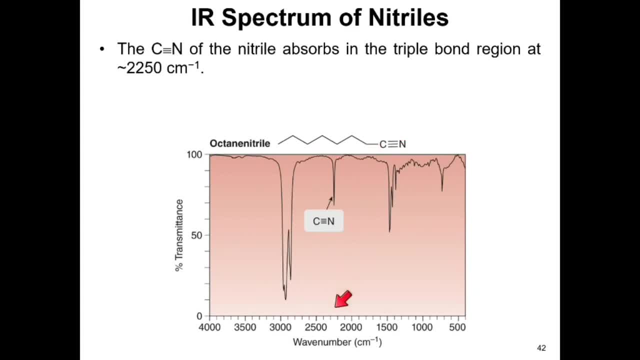 has an absorption at about 2250 wavenumber, And so octane nitrile has absorption in this region as well as between 2800 and 3000 wavenumber, due to the presence of sp3, hybridized carbon-to-hydrogen bonds. 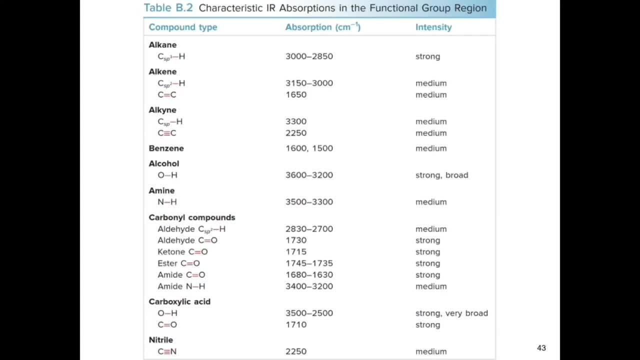 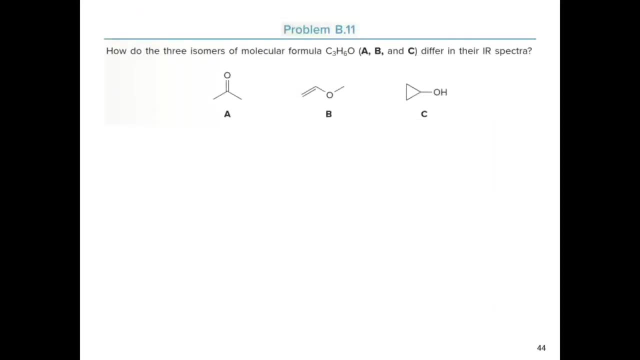 So here's the table that basically summarizes the different characteristic IR absorptions in the functional group region. And here's practice problem number 11.. How do the three isomers of molecular formula, C3H6O compounds A, B and C differ in their IR spectra? 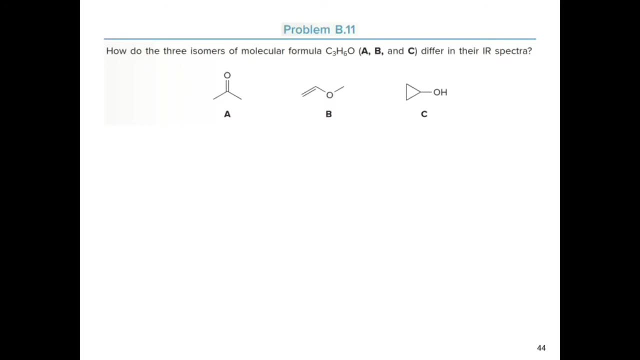 So for the first molecule here, molecule A contains a carbonyl group, and so you would expect an absorption around 1700 wavenumber, And in addition, this also contains sp3- hybridized carbon-to-hydrogen bonds- and so you would expect an absorption. 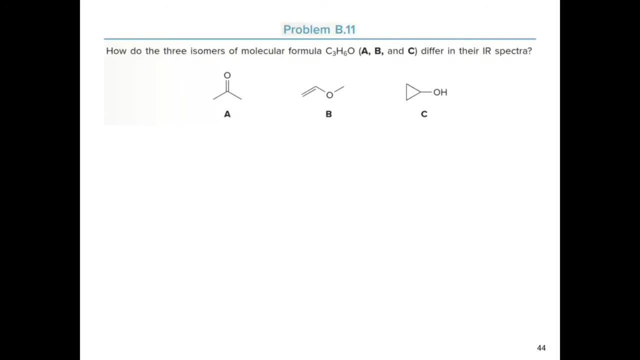 between 2800 and 3000 wavenumber. And for the second molecule, here we have a carbon-carbon double bond and we also have sp2 hybridized carbon-to-hydrogen bonds, as well as sp3 hybridized carbon-to-hydrogen bonds. 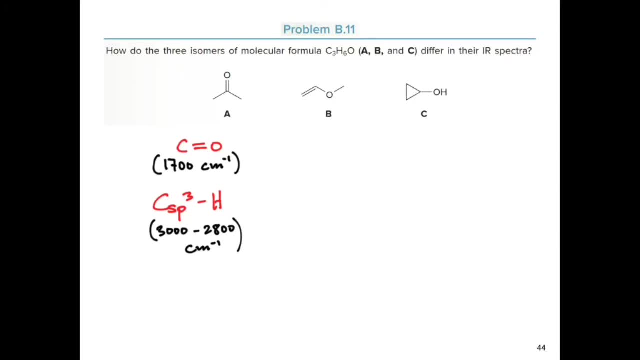 And so you would expect roughly three major absorptions. So again one around 1650 for the carbon-carbon double bond, And then we have the sp3 or sp2, hybridized carbon-to-hydrogen bonds, which occur at about 3100 inverse wavenumber. 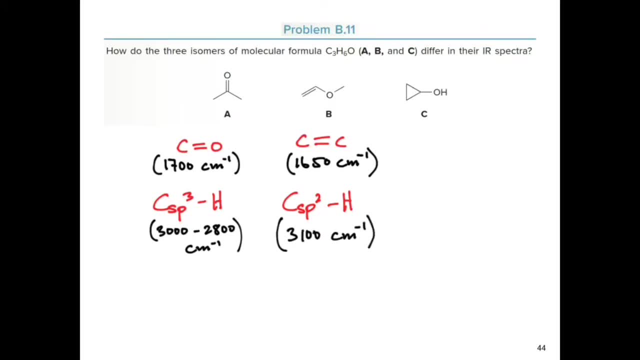 And sp3, hybridized carbon-to-hydrogen bonds, which occur between 2800 and 3000 wavenumber. Alright, and for molecule C, here we have a hydroxy group which occurs between 3200 and 3600 wavenumber. 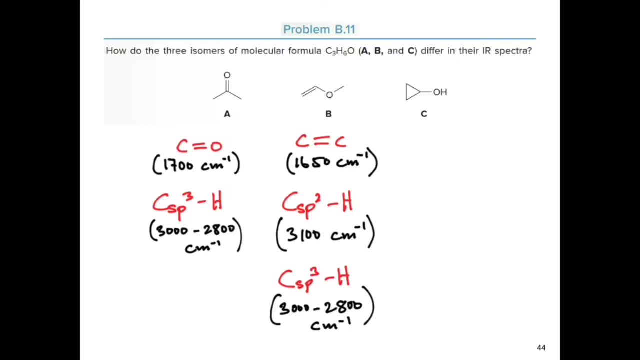 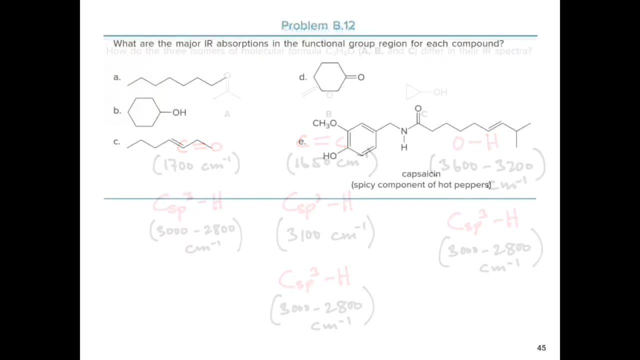 So you'll have a broad absorption around that region And, in addition, you're also going to have absorption between 2800 and 3000 wavenumber Due to the presence of sp3- hybridized carbon-to-hydrogen bonds. What are the major IR absorptions in the functional group region? 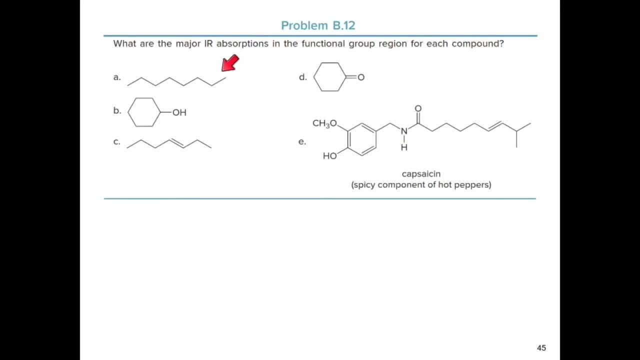 for each compound. So for the first compound here you can see that we have an alkane, And so the only IR absorption here occurs between 2800 and 3000 wavenumber due to the presence of sp3, hybridized carbon-to-hydrogen bonds.